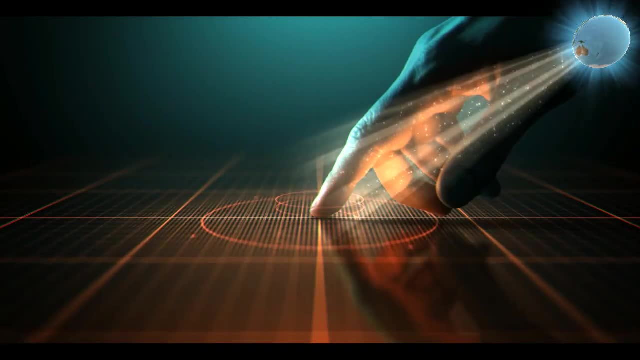 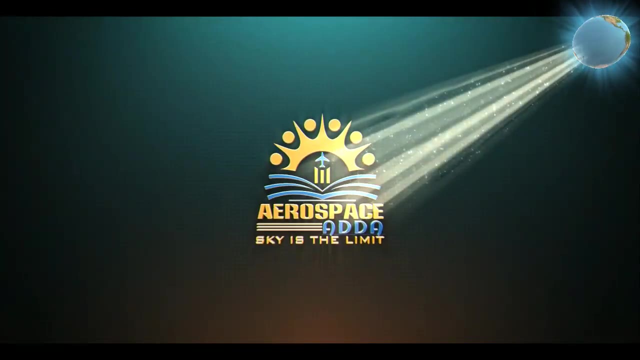 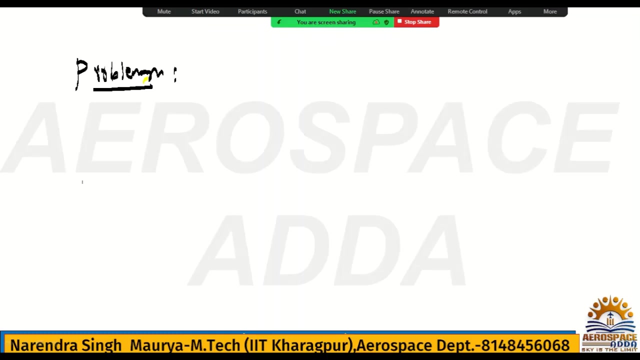 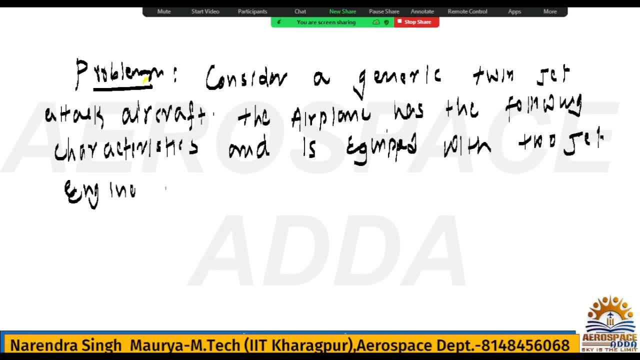 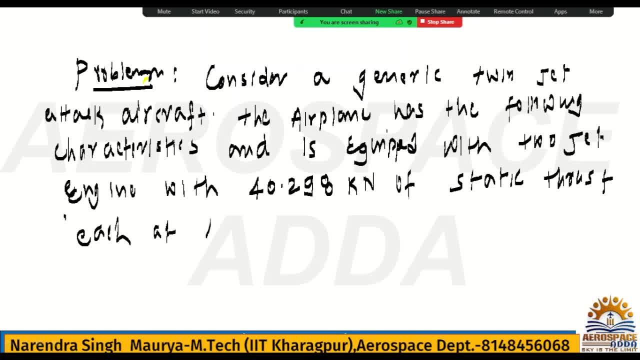 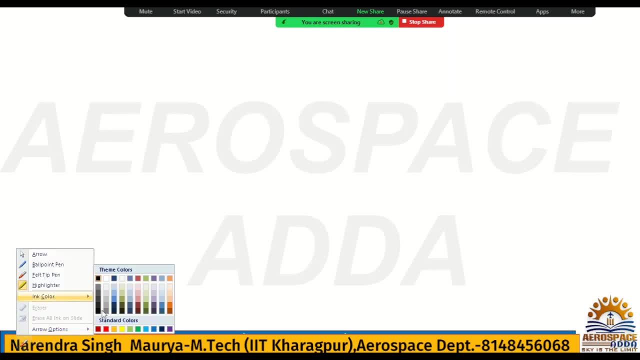 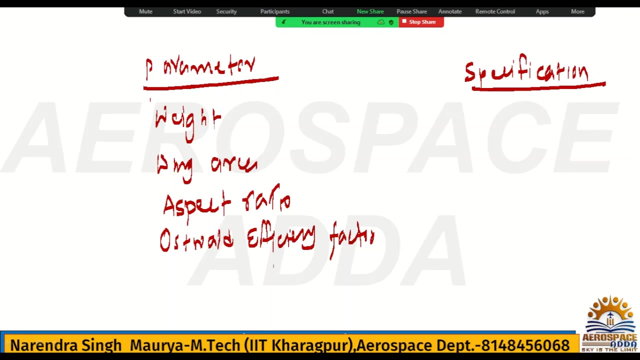 this is the a parameter and here we have specification, yes or no parameter and specification. what is that check parameter? here it is given weight parameter, here it is given weight parameter. here it is given weight, then v area, then stack ratio, then post wall efficiency factor. okay then. 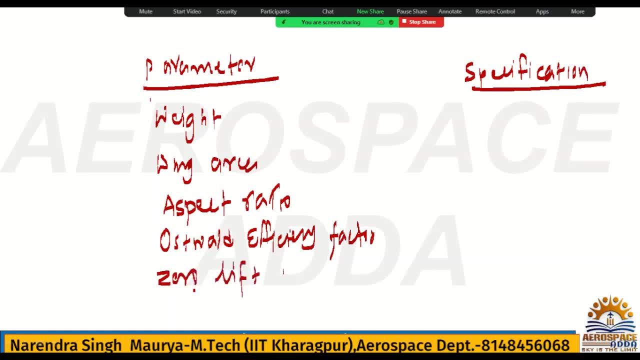 they have given zero. they have given zero, they have given zero lip drag. oh, it is here. write down the given specification here. write down the given specification here. write down the given specification here. it is uh weight is. it is uh weight is. it is uh weight is one zero three. 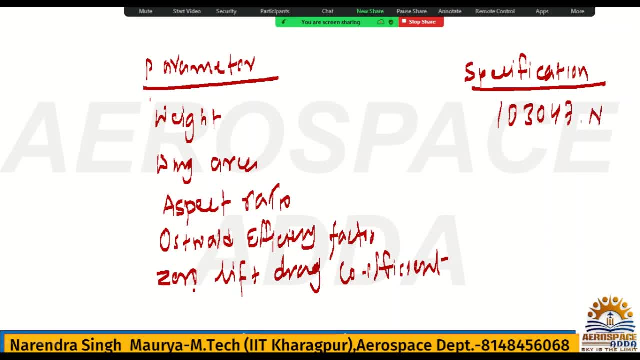 zero four, seven, newton. once again i have to zero three, zero four, seven, newton. once again i have to zero three, zero, four, seven, newton. once again i have to check one zero three, zero four, seven. check one: zero three, zero, four, seven, newton. check one: zero three, zero, four, seven, newton. area of the wing they have given. 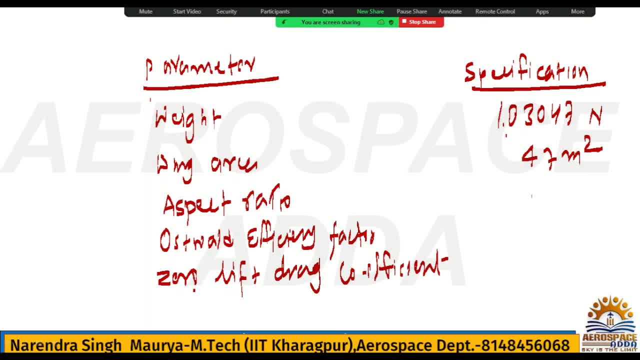 area of the wing. they have given area of the wing. they have given 47 meter square, 47 meter square, 47 meter square aspect ratio. they have given 6.5 aspect ratio. they have given 6.5 aspect ratio. they have given 6.5 okay. 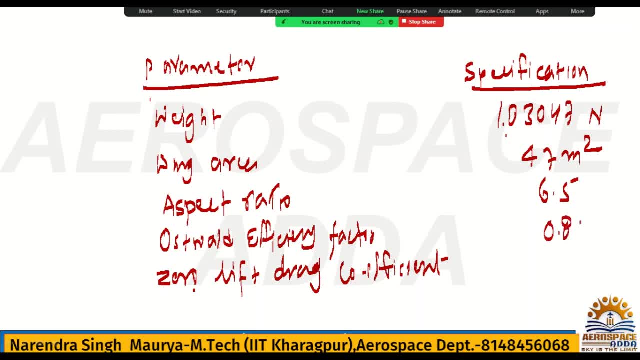 okay, okay. those qualifications, they have given zero. those qualifications, they have given zero. those qualifications, they have given zero point point. point. zero point eight. seven. zero point eight, seven. zero point eight seven. zero left drag coefficient. they have given zero left drag coefficient. they have given zero left drag coefficient. they have given zero point. 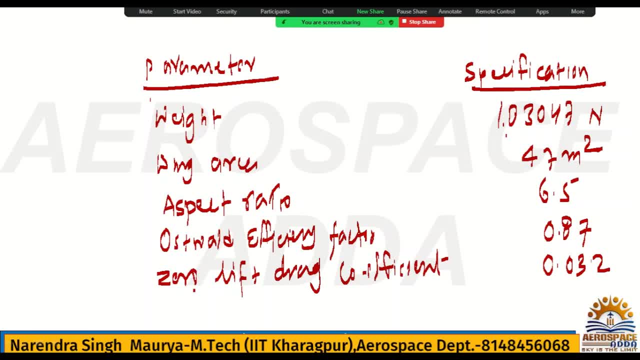 zero point, zero point, zero three, two, zero three, two, zero three, two. please write this. please write this. these are the specification means given. these are the specification means given. these are the specification means given: data okay, data, okay, data okay. these are the given details. these are the given details. 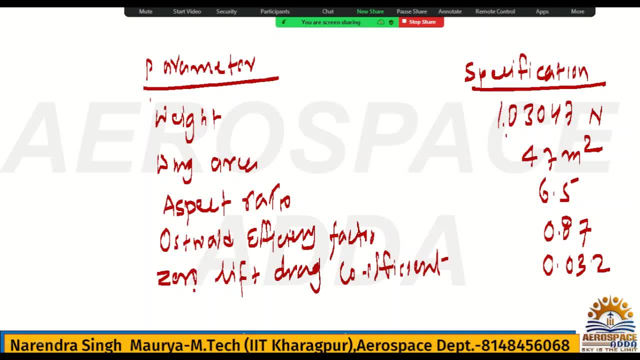 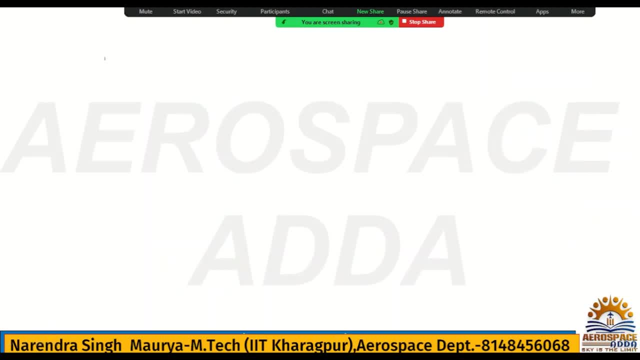 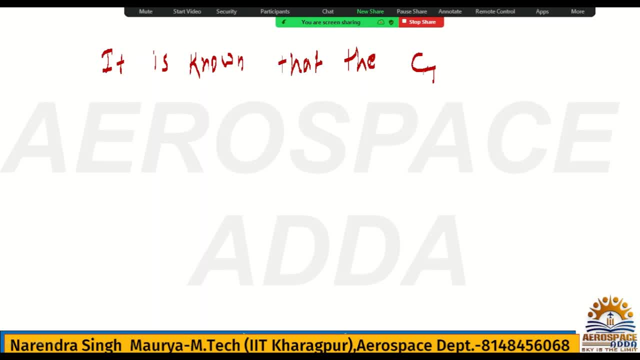 that the specific thrust fuel consumption means, means, means ct. what is the ct? it is the ct. what is the ct? it is the ct. what is the ct? it is the specific thrust fuel consumption. they have specific thrust fuel consumption. they have specific thrust fuel consumption. they have given in wording, they have given. 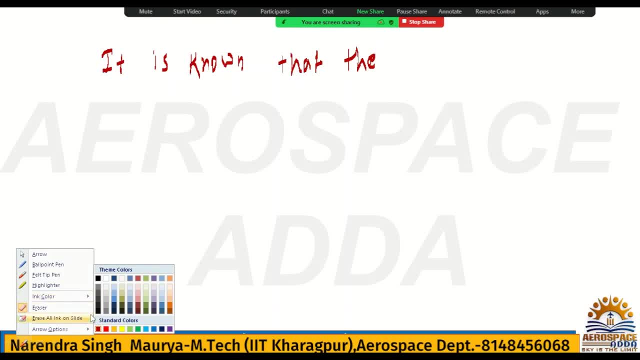 given in wording. they have given, given in wording, they have given, okay, what they have given, what they have given, what they have given. it is known, the specific, it is known the specific, it is known the specific, the thrust fuel consumption they have given in the, the thrust fuel consumption they have given in the. 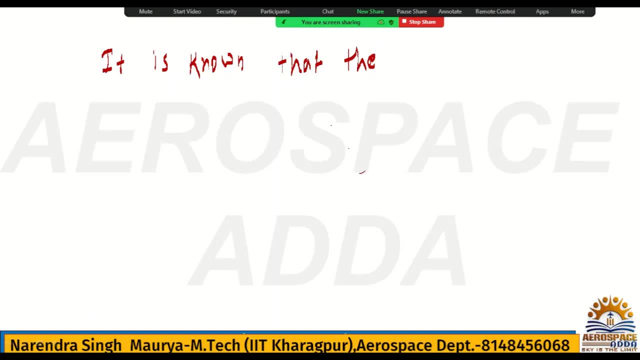 the thrust fuel consumption they have given in the the first specific fuel consumption, first specific fuel consumption, first specific fuel consumption is one newton. one newton, one Newton of fuel, of of fuel of fuel per Newton of, of thrust per check the unit what 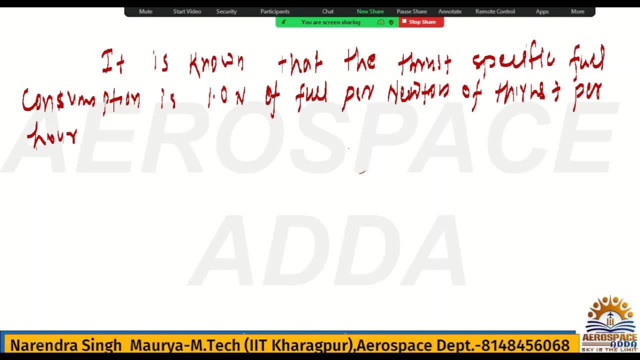 they have given. you have to change accordingly. okay, thrust per hour. right, the fuel capacity is. the fuel capacity is whenever you are going to fly, then what is the fuel capacity? that is nothing but, or fuel capacity during takeoff. you can say the fuel capacity is. 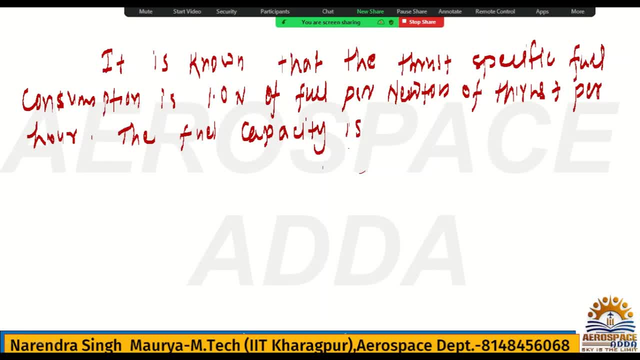 is is 57,. how is the Newton? this is the amount of the fuel. okay, fuel capacity, and remember this fuel capacity means what it is during the takeoff. it is during the takeoff, okay, 57,000 Newton. the fuel capacity means whenever that aircraft is what going to fly that time. 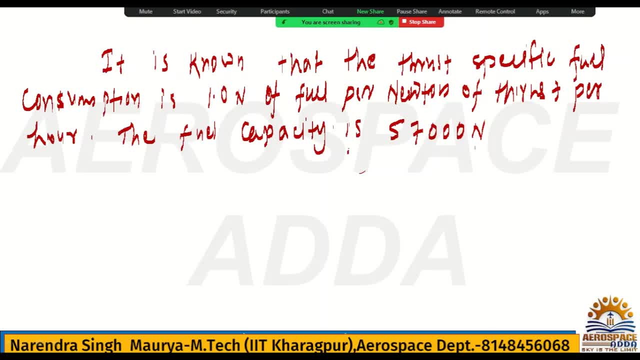 aircraft you are carrying the amount of fuel. what amount of fuel? 57,000 Newton, this thing all right now. and and maximum, maximum gross weight is 136960 Newton. Just think this is the amount of the- I mean weight of the aircraft when it is. 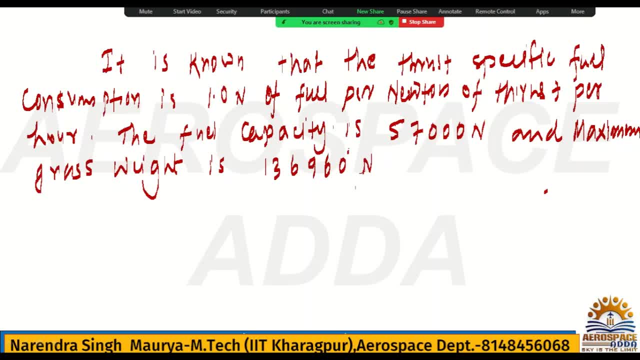 going to fly. gross weight: maximum gross weight. calculate full stop, no, calculate the range. range and endurance. this is the finest and lengthy numerical. if you able to solve this, then your range and endurance problem, I mean, you will able to cover all type of what type? 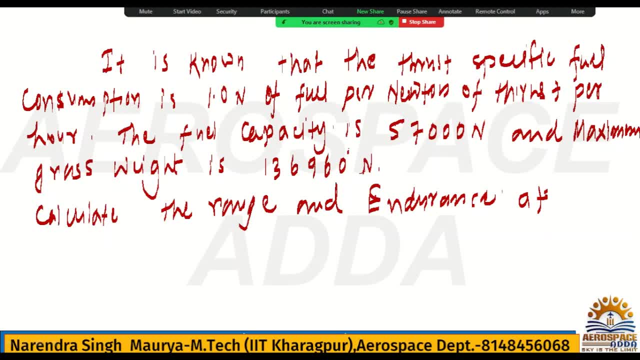 of question they can ask in different, different unit. now, if you solve this, then you may understand clearly. endurance at a, at a standard, at a standard altitude of 8 kilometer, ok, ok, ok, at 8 kilometer. this is the problem, yes or no? this is the problem. so you read it first again one more time. you read: check what question? 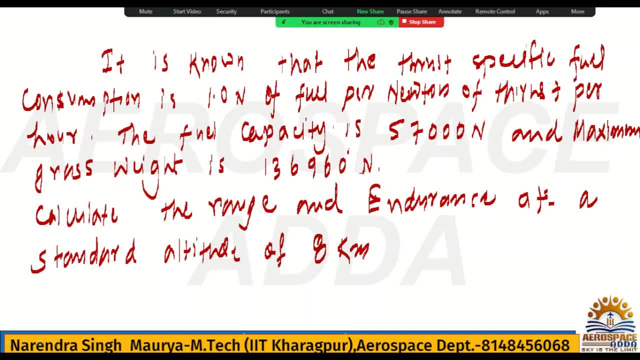 they are asking- that is the important point, yes or no? existe esto no range endurance. they are asking to calculate. Very importantly, you need to check. this is what: this is the jet engine or propeller engine, propeller powered engine? yes, this is the jet engine, because thrust they have given. they said this is the in problem of the, the range. 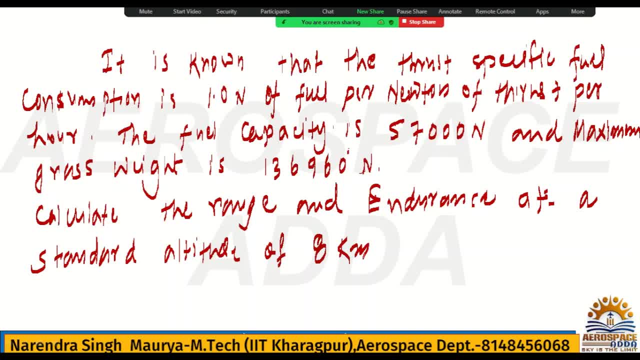 like amount of the seam. read from the starting they had given two jet engine and static thrust. for that they had given. so overall, you got the idea. okay, this is what, uh, i mean jet engine. so, for jet engine, okay, write down option. write down option for this problem. this is the problem, this. 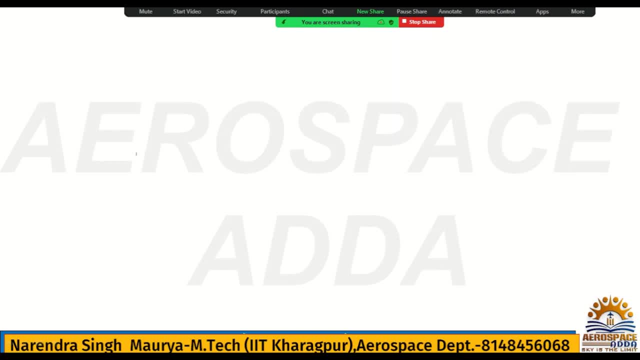 is a lengthy one, okay, but anyway you able to solve them, it is fine for you. a range: they have given to you two seven seven zero kilometer, and endurance: they have given to you three point eight, two hours. option b check range is given two, seven, seven zero kilometer. 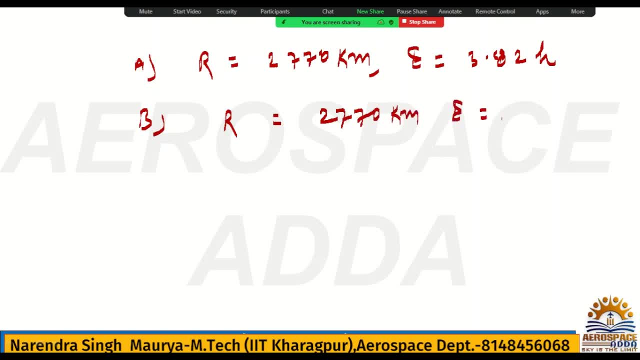 and e. they have given to you how much it is: 6.33 hour option c range. they have given to you how much four, two, five, zero kilometer and endurance. they have given how much three point, eight, two hours option d range. they have given four to five zero kilometer and endurance how much. 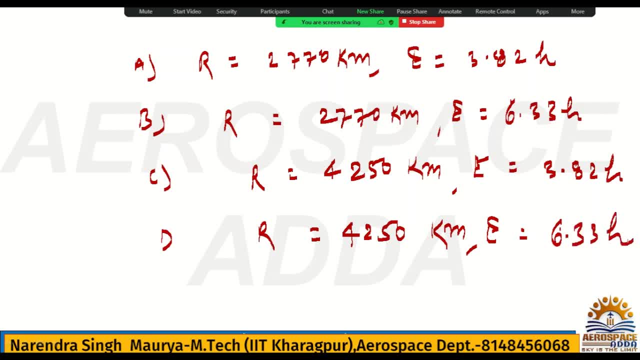 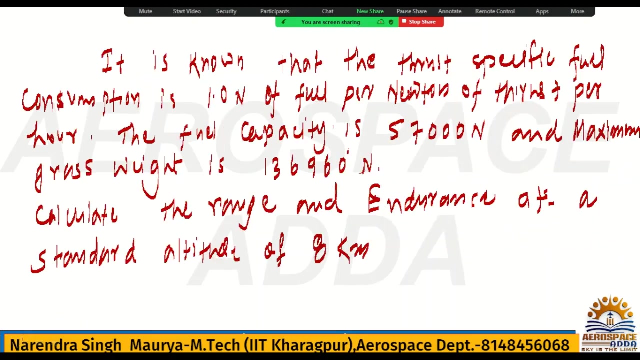 six point three, three hours. please make a note of this. it's a nice question, nice question. check all the data, what they have given to you, yes or no? check what they have given to you, all the data, all right now. so let me circle the important part here. so, because this is the general information, 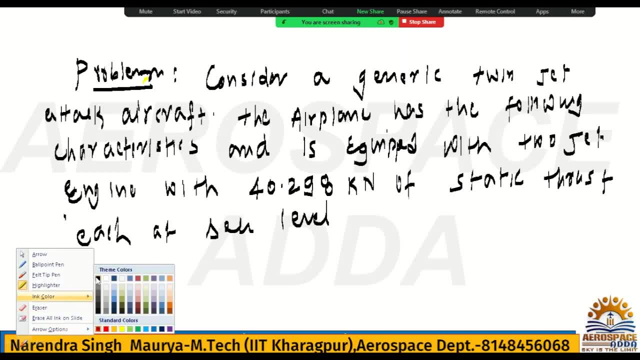 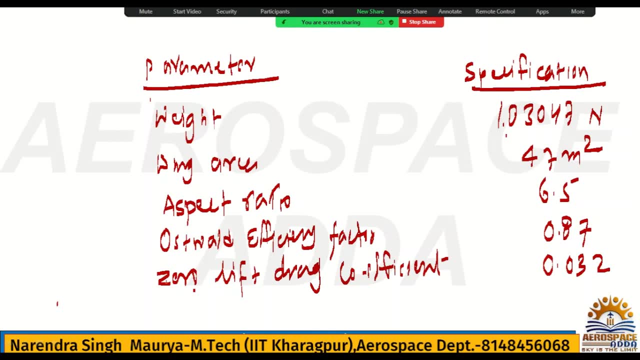 for the aircraft they have given to you. now, for the aircraft they have given like generic specification of the jet attack aircraft and what important point here- that weight, okay, big area- they have given to you four, seven meters square respect ratio or small efficiency factor, zero lip drag. so this is the information they have given to you. 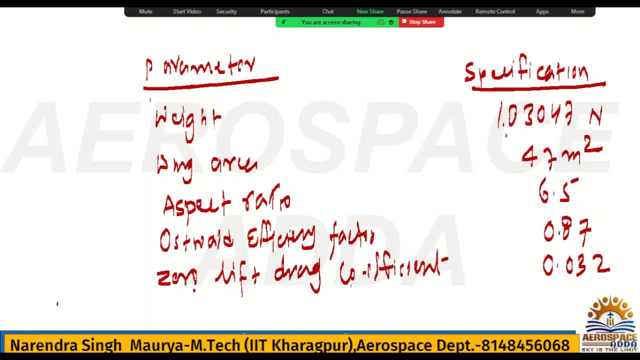 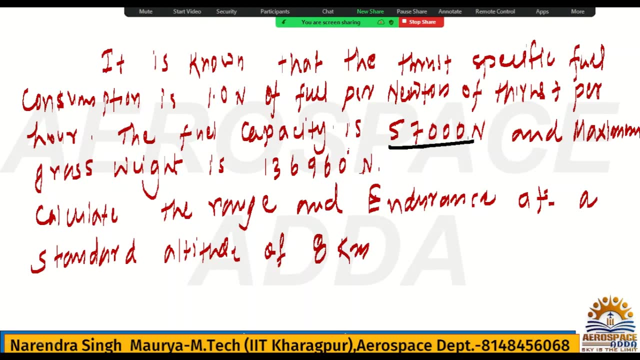 yes or no. now we'll go for the next part. what they said. check that fuel capacity. they have said it is 57 000. okay, it is 57 000. they have given the weight of the fuel means. what means wf, w capital, f, or you just say fuel, better, f? u, e, l fuel. what is this gross weight? they have said means? 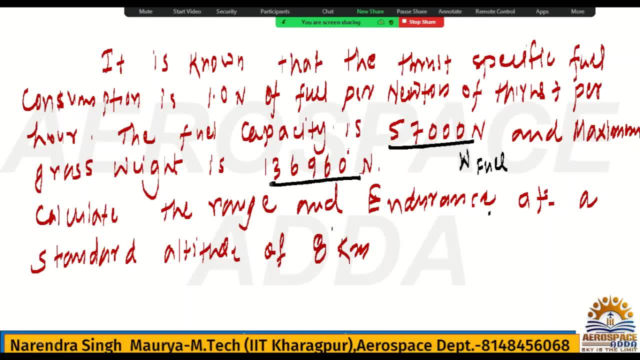 when it is going to take off. so maximum gross weight means it is the initial weight. so in our formula it is w naught check. it is w naught yes or no. yes or no at eight kilometer. that aircraft will not fly at air get kilometer. that is one very important point. 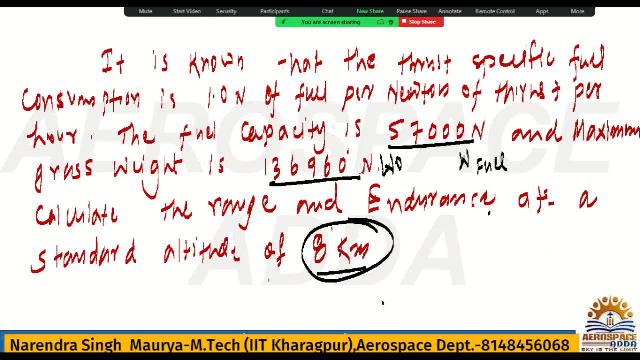 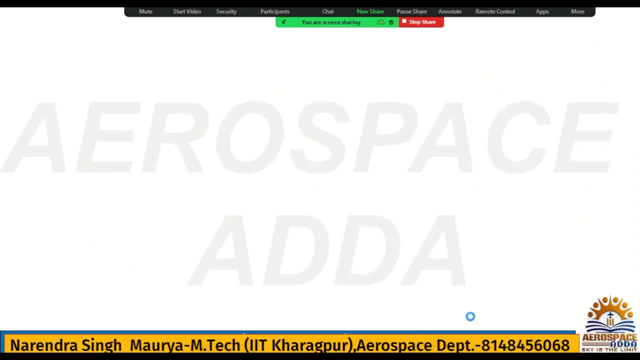 you need to remember because in formula uh, range and endurance formula, if you are using and if there is a density, so density, you have to keep at eight kilometer. that is the one clue. it is very important now remember. okay, now, range and endurance, so we'll proceed. this it is very simple one, but anyway. 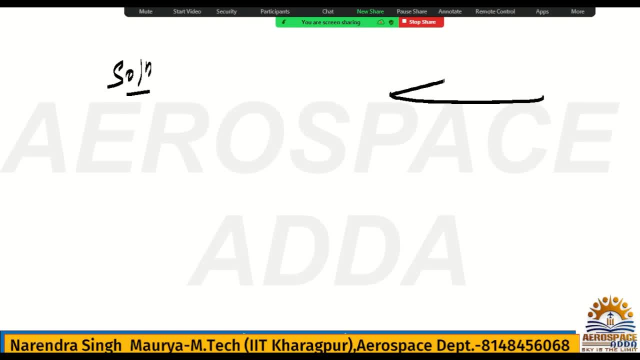 check that aircraft is what flying. okay, it is flying from c level to this altitude is nothing but eight kilometer. okay, so what will be the density at eight kilometer? you need to calculate first. okay, so that is the one part. you will proceed like this: th is nothing but t naught minus l h. t naught is what 288. 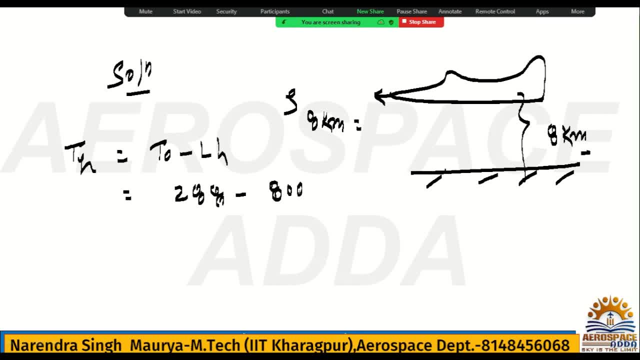 minus l is nothing but eight kilometer. so eight kilometer means eight thousand meter. uh l sorry, h is eight thousand. here i'm writing: l is nothing but zero point, zero, zero, six, five, click. this, is it okay? anyway, first i have written, no problem. where is my calculator? 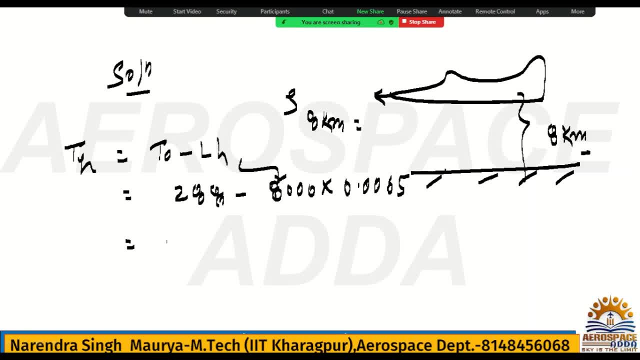 so this is nothing but 288 minus zero point zero, zero six five, okay, into eight thousand. so i'm getting 236 kelvin. okay, this is the th, fine 236 now, if i want rho, h by rho naught, so it is nothing but th by. 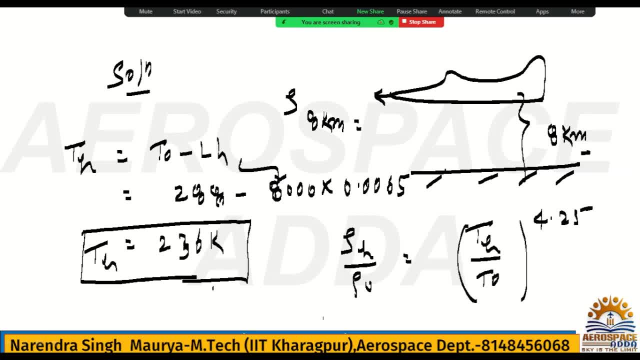 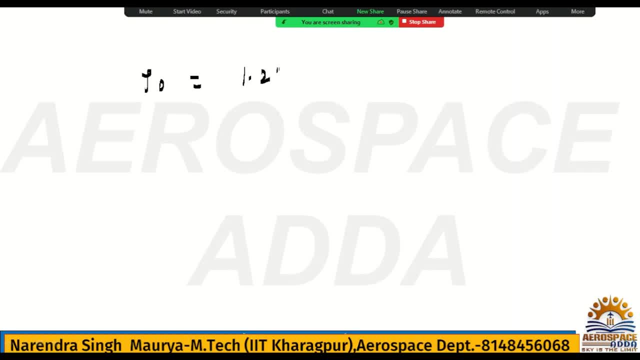 t naught two whole power: 4.25. what is the ro not row0 is the. what is the rho naught? rho naught is the sea level density: 1.22 kz per meter cube. so what is the rho h, which is nothing but rho, at 8 kilometer? what is that? it is nothing but rho naught. 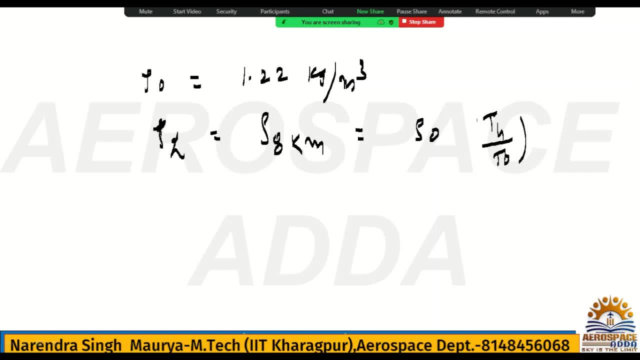 into th by t naught 4 power, 2.5, 4.25. yes or no, 4.25 now. so what is this value? check: 236 divided by 288 to whole power, to whole power, 4.25 into 1.22, right i am getting. i am getting 0.5 to the kz per meter cube. 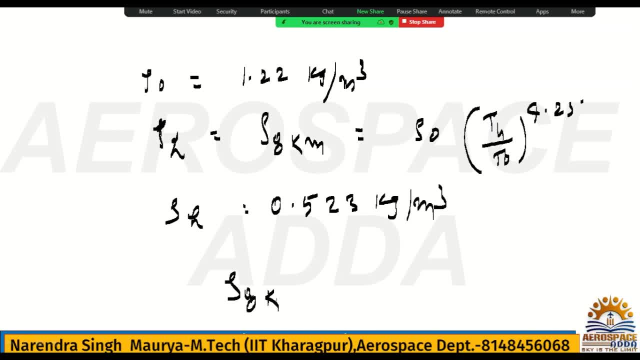 so this is the one thing. you got: density at 8 kilometer, which is 0.5. why i have calculated this? because i know that density term will come in range and endurance for the jet engine, yes or no. now we'll go further, because it is the jet engine, because they have mentioned. 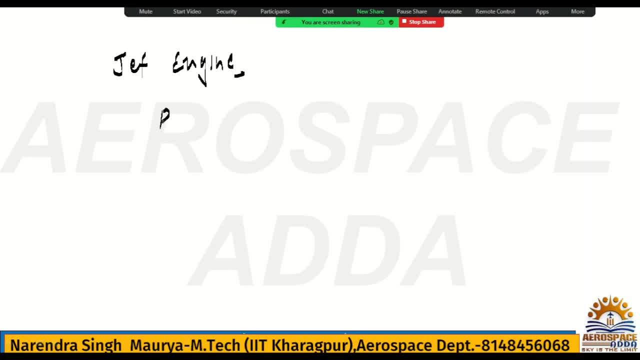 in problem itself. so for jet engine, what is the range formula? you check it. what is the? what is the formula for range and endurance? let me write this directly, because this problem should not take more time, so we can go for another problem also, yes or no. now check. so range is nothing but 2 upon tt. okay, and here it is. 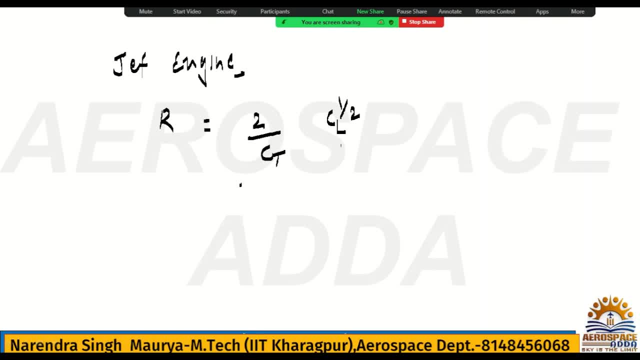 cl for jet engine, cl to power, 1 by 2 by cd, okay, and it is 2 upon rho s, okay, and which is nothing but w initial root, w final. all right. this is the problem, yes or no? so now, if you go for this, then 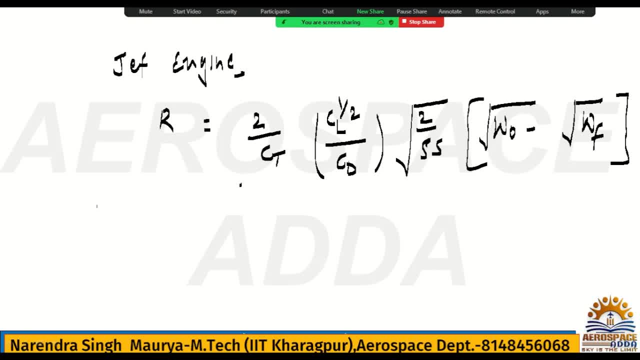 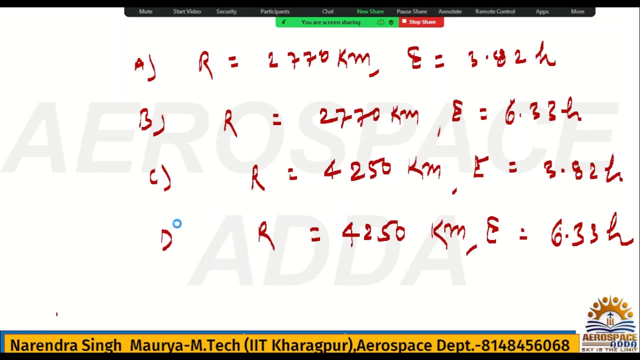 check tsfc, which is nothing but thrust specific fuel consumption ct. they have given to you, but it is not given directly, it is given in different way. what different way it is given that one newton check the statement, only you will understand it is given thrust specific fuel. 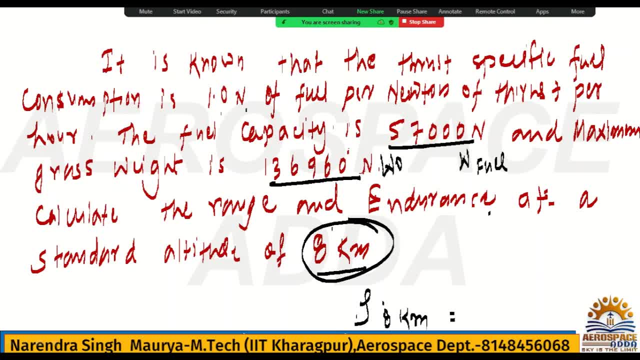 consumption. here thrust specific fuel consumption is nothing but one newton of fuel and it is given, okay, per newton of thrust per hour. okay, it means ct. they have given in this format check they have per hour. okay, it means ct. they have given in this format check. they have said one newton, one newton. 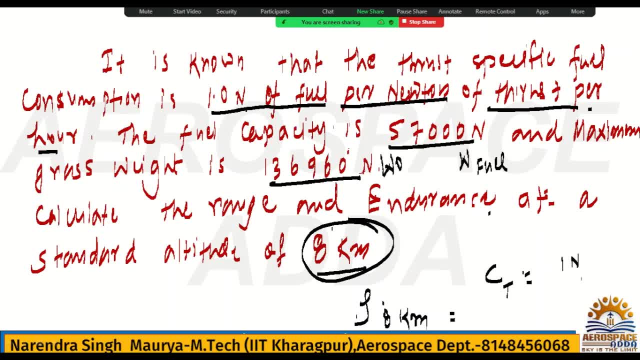 one newton of fuel per newton of thrust. thrust per for newton of trust per became. thrust per hour means by hour. this is the mistake. we are not satisfied when we say ct, for how much per hour hot fuel occurs? rush queria for 14.85. we cannot see any and would say 1 hour. and imagine car horns. it does not matter since we had three engines. orАst破押ius9. 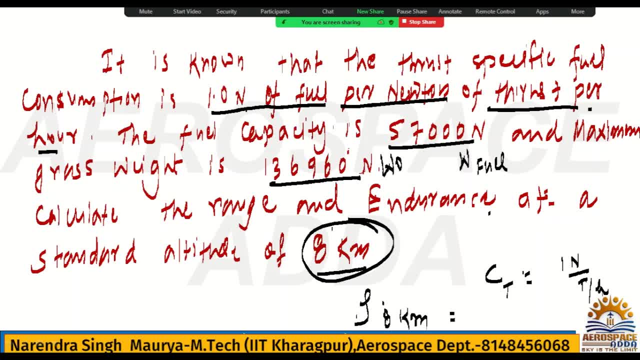 this is the value they have given. so basically, it is given- uh, you can say, it is given- one newton divided by newton hour that you can write. that you can write because this you can run, newton per hour you can write and thrust is one newton. that is the one thing. so you just convert this. 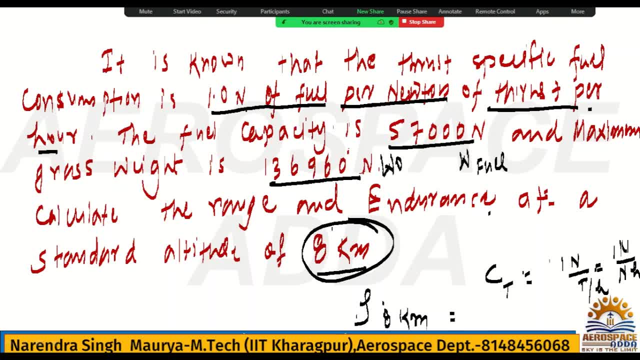 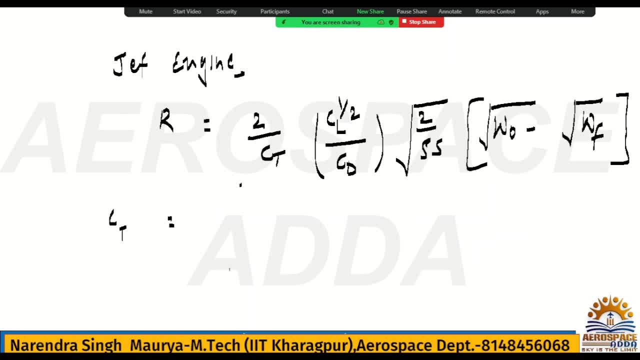 into one newton divided by newton second. so that will be the perfect unit, yes or no? so here you may write: ct is equal to what they have given you. read it, you will understand what unit they have given. your tshc, which is nothing but thrush, is basic fuel consumption. 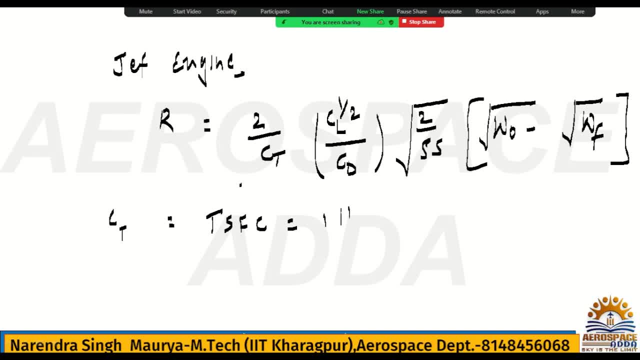 that is nothing but one newton divided by newton hour. you just convert it into second. so if you do, then do this, then what you will get: one newton divided by newton as it is, but hours you can write 3600 second. if you solve this, then what you will get. 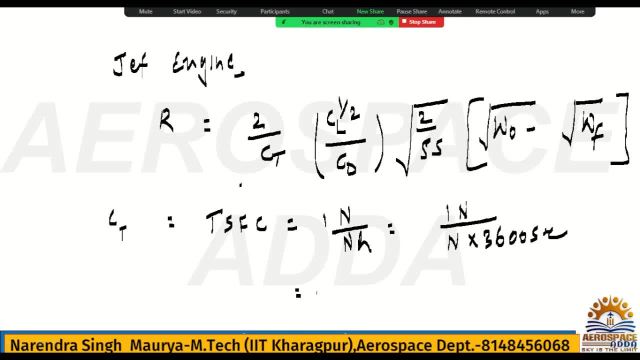 let me calculate one upon three, six, double zero. it is two point seven, seven, ten to power, minus four, minus four newton divided by newton second. now you unit is perfect. i mean you can use this. this is the ct. okay, this is the one thing. second thing: what you want, check in the problem. 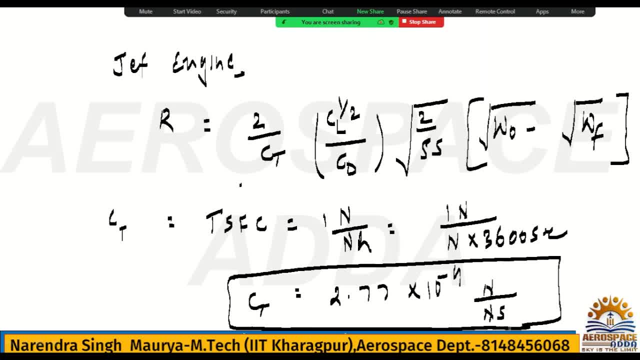 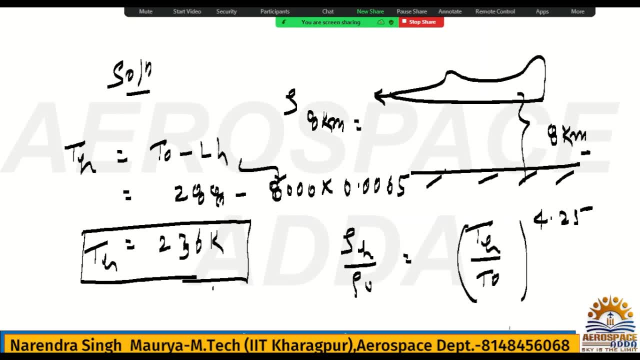 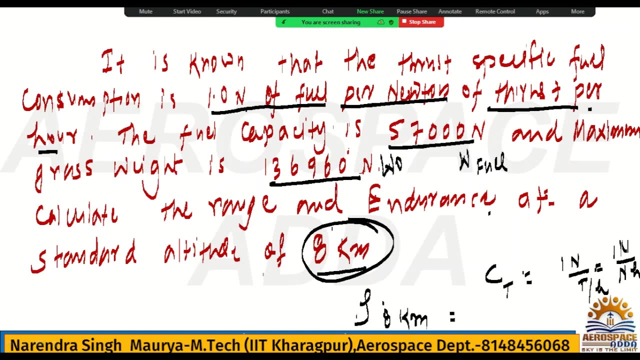 in this problem, even though they have not given, uh, that they have given the condition, but the specification they have given. but they have not mentioned anything like calculate the region in endurance, that is, standard altitude. so they have not mentioned any condition like maximum or maximum range and endurance condition like that. they have not given yes or no. now so, but check the. 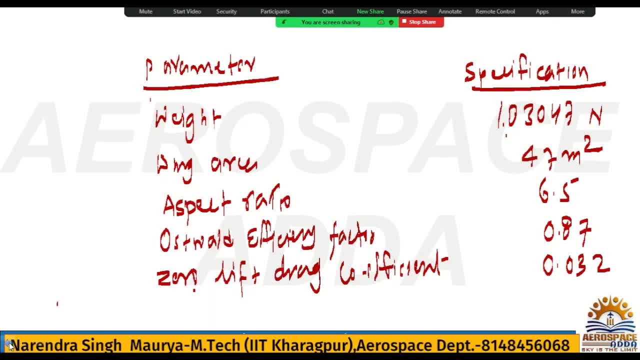 given data, what, given data they have given, based on that it is possible to calculate like clcd value, because root cl is there, yes or no, and how to calculate that uh root cl, that is the one, uh cl by cd, root cl by cd. how to calculate that? that is the one point. so if they have not given, then what you? 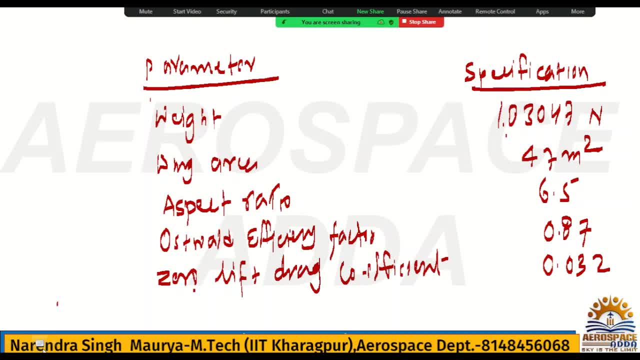 will do, because cl means what? if you want to calculate cl, then they should do velocity of the aircraft or anyhow they they should give the value. but if they have not given what they have given, they have given zero. lift drag coefficient means they have given cd, not what is the ocean. 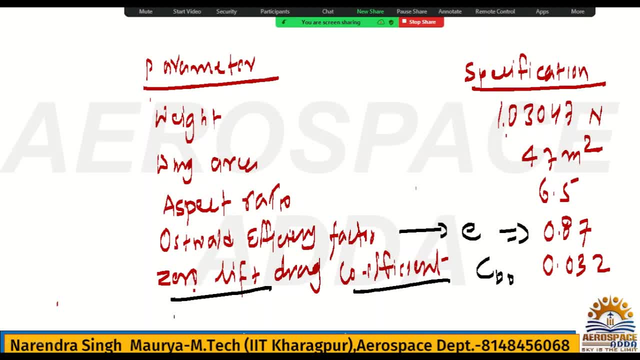 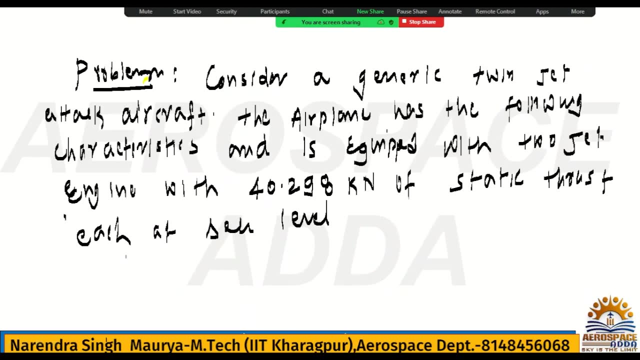 elephant celsius, it means it is e. so if and what is this aspect ratio here in? and they have not given any like uh, uh, you know the velocity, they have not given. so you cannot calculate cl value coefficient, you cannot calculate directly. okay, fine, so in this situation, what you will do, 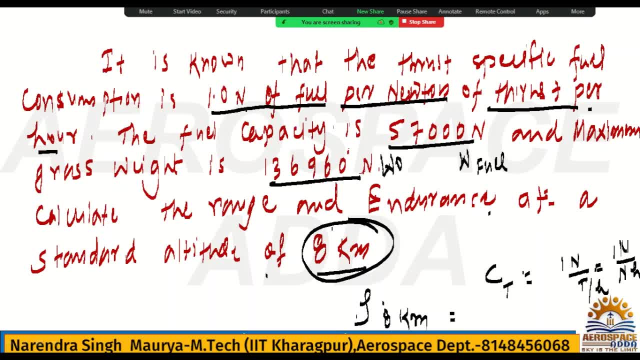 okay. so like, if you read the problem, because most of time they will do like this, read the problem. if you are not able to understand, like, okay, how to build velocity, uh and what, what should be the velocity and what should be the cl. if they have given cd not and all, so cd not, why they are giving cd not. that is the one. 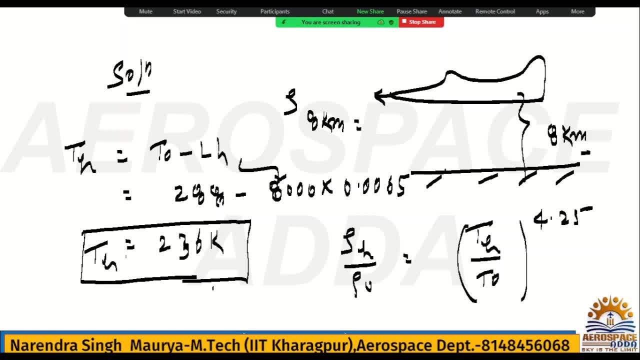 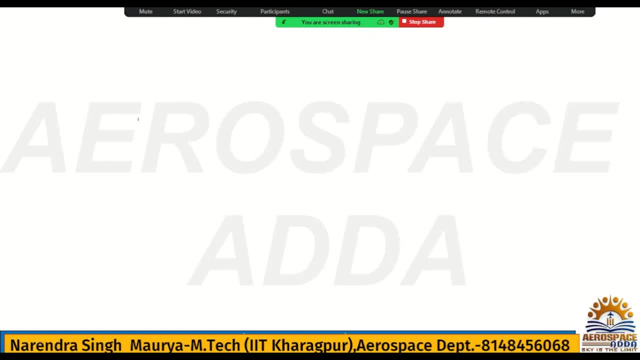 very important thing because if you check the formula range formula, that cd not is not required here, is it not required? similarly, if you write the endurance formula also, what is the endurance for jet engine? if you check the endurance formula also, see the endurance also, they have uh, endurance. 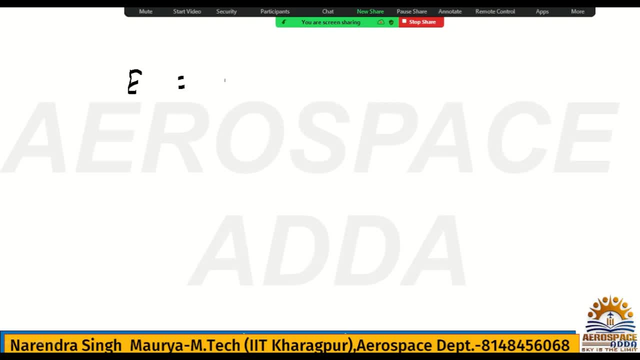 formula also that cd not is not required. what is the endurance formula? it is one upon ct, yes or no, and it is t, l by cd, yes, ln, ln. it is nothing but w naught by wf, yes or no. so if you say that, that meaning is very clear. they have not given the like condition. what condition? 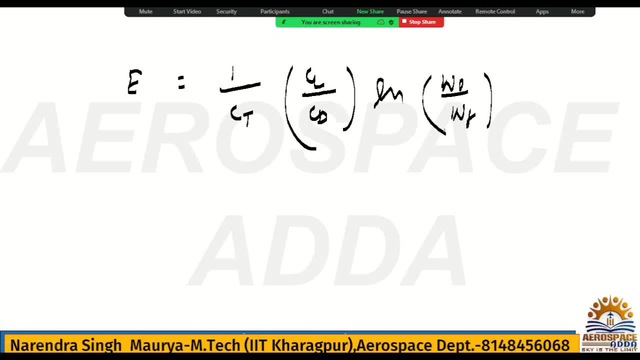 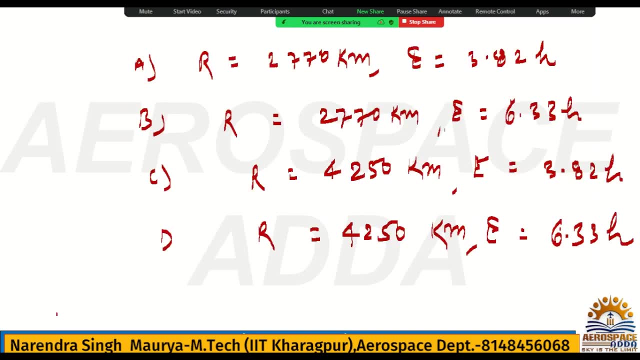 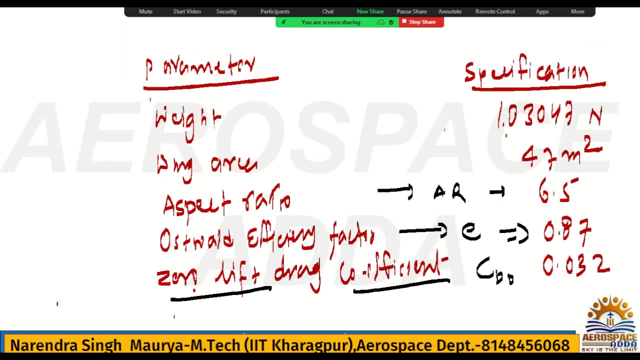 they have directly. they have not asked to you what is the maximum range and what is the maximum endurance. but you need to think why? because they have given the data. what data they have given? they have given, uh, this value, cd naught. they have given post hole efficiency, they have given a spectra, they have given, but 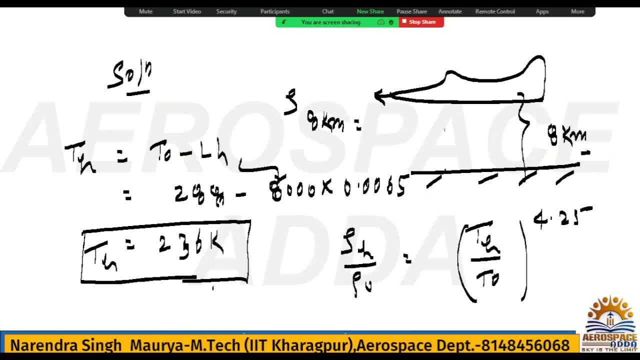 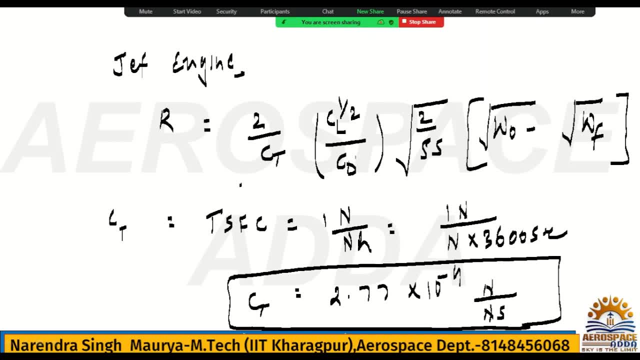 these value they have given to you, but you in the in the formula. if you check in the formula cl power 1 by 2 by cd, it means cl and cd. you are not able to calculate directly cl by cd here. also required that you are not not able to calculate cly because cl if you 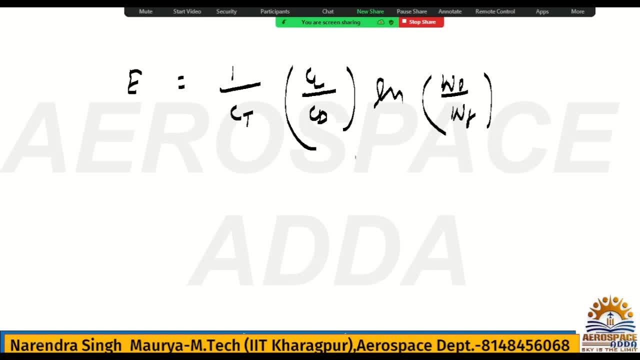 want to calculate, then you should have velocity, okay. so that time you need to think about cd, naught e and aspect ratio, when it will be used, when there is a condition, what condition? that maximum. so you need to. this is the node point. you also have to think in this way. 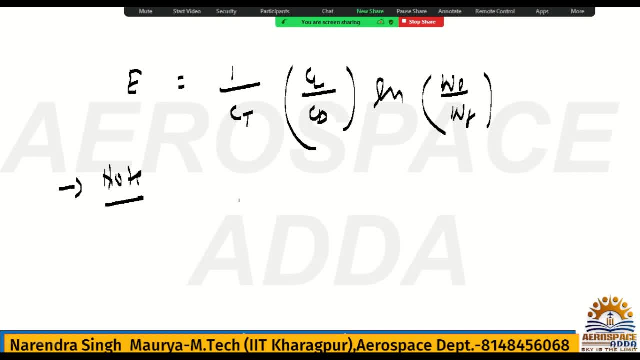 in exam. suppose question will be asked like this. then you have to write here: consider, consider the, consider the maximum range and extra means for endurance. then you have to actually calculate this problem. calculate this and then you will get the rate of their maximum. you will also get the number. 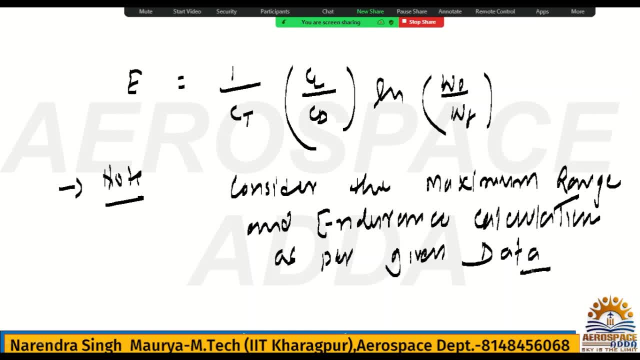 in details. then you will also have to take the c? l when it will be used. you have to do the Gaussian of finds to calculate calculation, shall or shall. and i say you have to use for maximum decaj. then the difference will be like z, which means you multiply it so that you can separate. 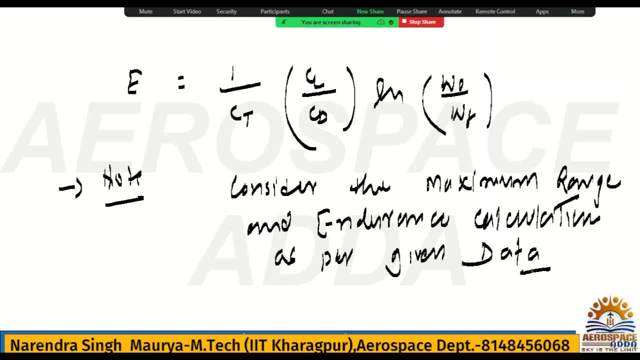 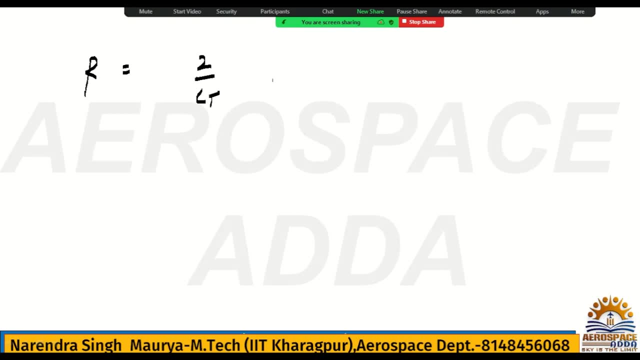 aspect ratio, yes or no, i know. school efficiency yes. so first we'll go for the range. what is the range range? check race formulae. to check, it is nothing but 2 upon pt and cl by cl power, 1 by 2 by cd, okay. 2 upon rho s, yes, in bracket, initial weight w naught, minus final weight w remember. 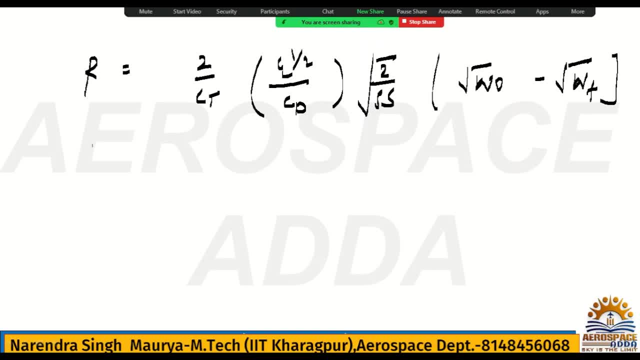 this is not a fuel, this is the final. okay, how to calculate final, final, if i should write final, otherwise you may get confused because fuel and final student may get confused. what is the final? so final is nothing but initial weight w naught minus what amount of fuel you have burned. if you remove that, what amount of? 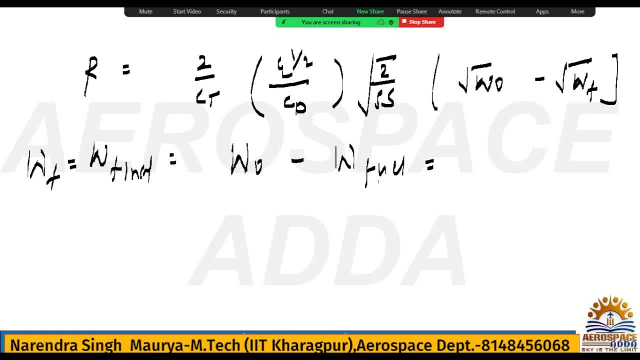 fuel you have burned. if you remove that, then you will get the final wf. now what is the check? initial weight they have given to you? okay, let me check my pdf to better, because again and again I'm going back. so that is not good now. so initial weight is nothing but one, three, six, nine, six. 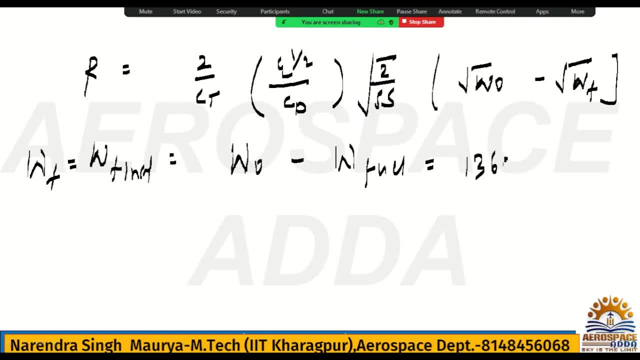 j, zero, yes or no. one three six. one three six nine six zero. this is the initial weight minus what is the final weight you had calculated it was, it was given 57 000.. check that problem, read it now so you will get so. what is the final weight if you calculate? 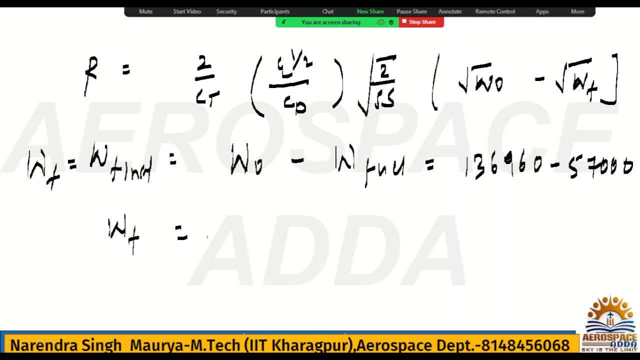 w final. so let me write one three, six, nine. one three, six, one three, six, nine, six, zero minus minus five, seven thousand. so you are getting seventy nine, seventy, nine, nine, sixty newton, seventy nine thousand, nine hundred sixty newton. this is the final weight you are getting. 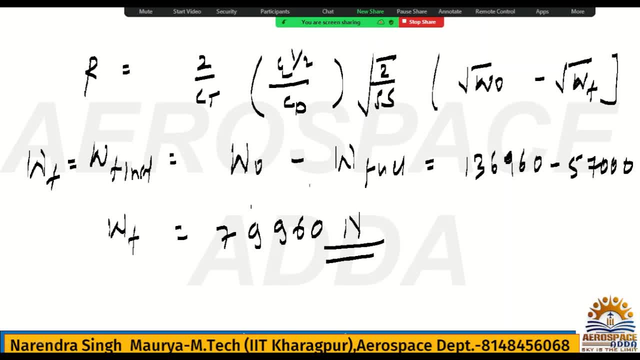 now you use that. what is the value of the cl to power 1 by 2 by cd maximum, because you are, you have considered range max and endurance max also. so for that, what will be the formula? two upon ct, yes, or no, two upon ct? cl to power 1 by 2 by cd. 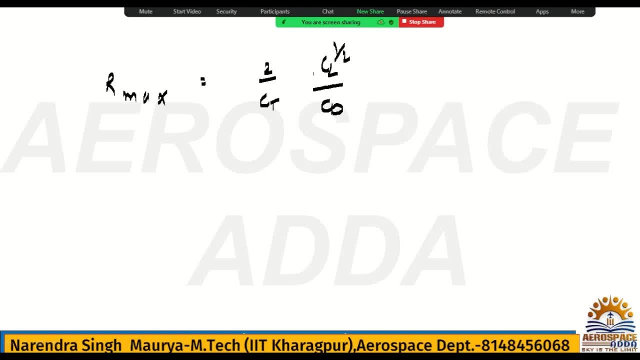 yes, cl2 power, 1 by 2 by cd and this is the final weight in e cuid should be maximum. okay, check the jet engine range. how to calculate this maximum cl? uh, that we had seen that minimum drag condition, minimum power condition and minimum thrust to velocity in that. 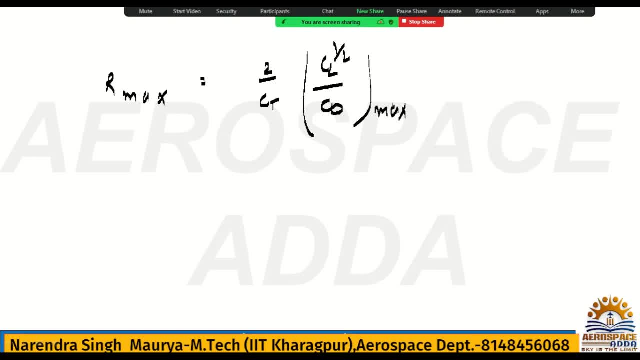 cl power 1 by 2 by cd. we had calculated that time. you please go back and check it now. so so you may get two row s, remember. this row is nothing but at eight kilometer, and here we have initial weight weight. this should be separate now. so i am going slow, because last class we had seen that numerical. 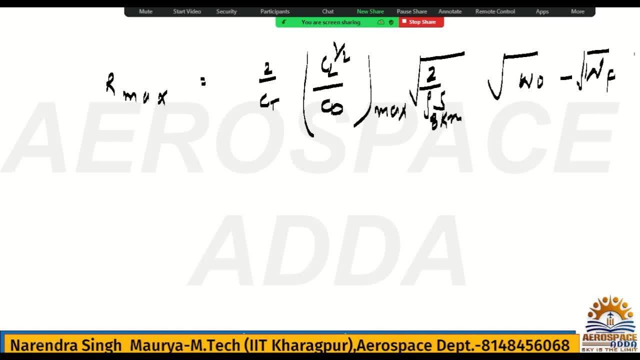 in the numerical. we were not getting answers, so better we'll go slow and calculate properly. fine, so how to calculate cl to power 1 by 2? it is given in your notes already. i had calculated that thing first. this is the condition when thrust by velocity. 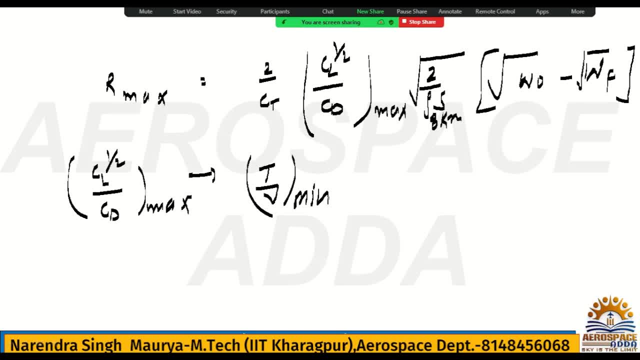 should be minimum that that we had seen, or maximum that we had seen that we had seen. if you go back and check it so you may be able to understand how to calculate a cl uh, cl by cd, cl power, 1 by 2 by cd max, how to calculate so. 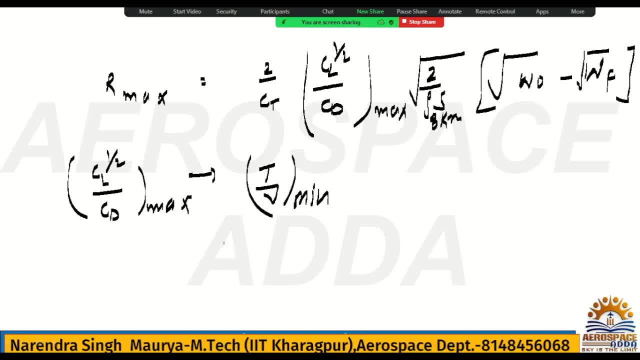 yes, if you remember, it was thrust by velocity minimum. what was the formula it was? it was anyone. do you remember that it was crushed by velocity minimum if you go back and check the nodes. so this is the condition where you will get 3d, not 1 by 3. 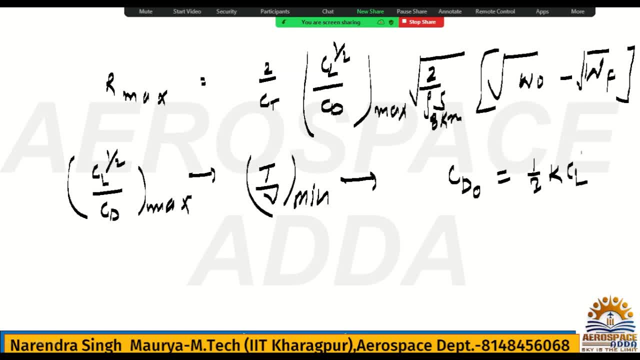 kcl square. this is the condition you may get now. if you check, please go back, check in your notes. it is properly derived for that reason. uh, that time i had derived because i told you that time this will be used many places. okay, so cd 0: 1 by 3 kcl square: yes, now, so if you calculate what is the cl. 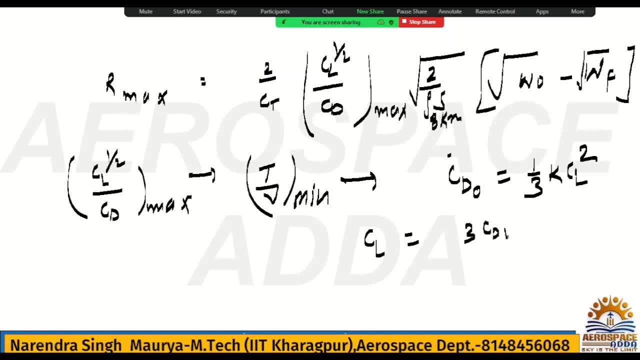 what is the cl, so it will be. this is cd naught by is equal to 1 by 3, 1 by 3 KCL square, or I think it is 3.. Can you check that? Can you check that? once It was 1 by 3 or. 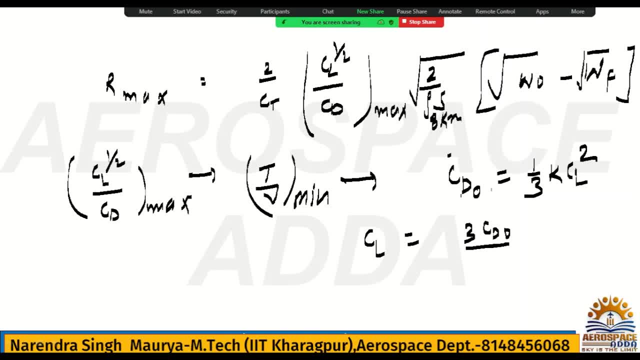 I think it was 3 KCL square. if I am not wrong, Then only if you calculate C D naught by 3 K root, C D naught by K, 3 C D naught by K. So I think it was 3.. Check it. 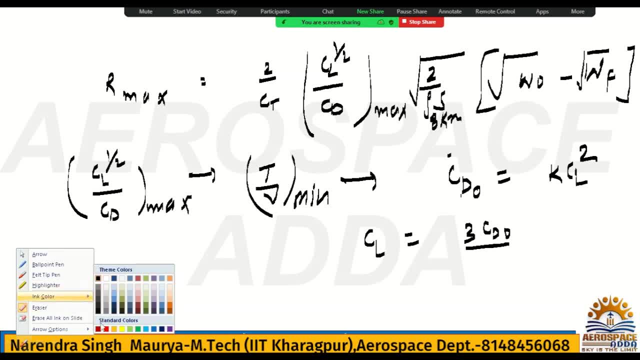 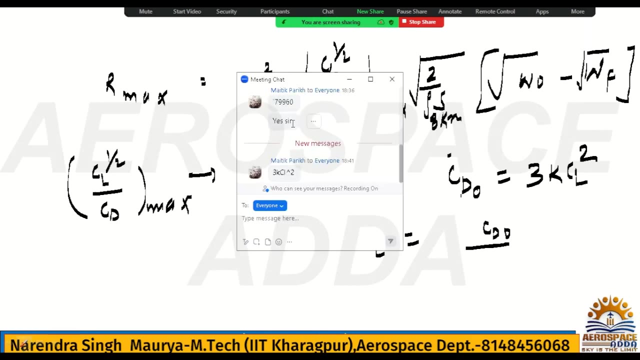 Take any words here please. Even I do not remember, because that is the formula. it was derived that time, So I think it was C. D naught is equal to 3 KCL square. So if you go for the T L value, Tell me somebody has 3 KCL. Yes, yes, very good, Thank you. 3 KCL square- Yes. 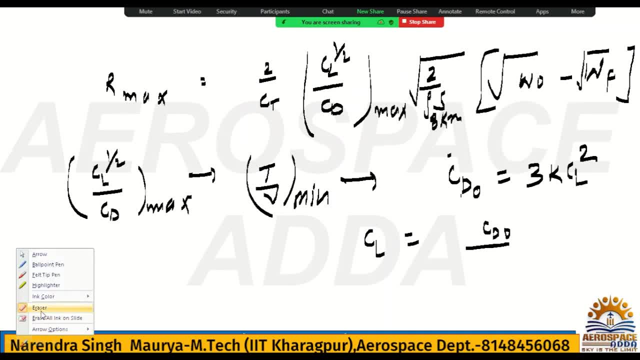 it was given in your notes. I had derived that. So it is sometimes confusing. So for that reason also I am telling to you: You remember the formula, because sometimes you know minimum power and this C, D naught, this thrust by velocity, conditions may like mismatch. So for that reason you remember. 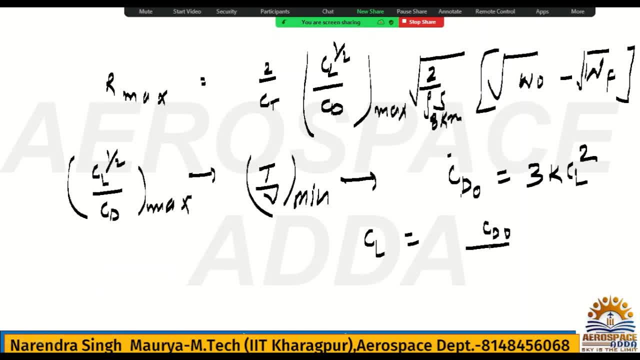 properly. So it is nothing but CD naught by 3k root. Yes, you calculate that value they have given to you. What is the CD naught they have given to you and what is the k? k is nothing, but you know formula 1 upon pi, e, a, r. 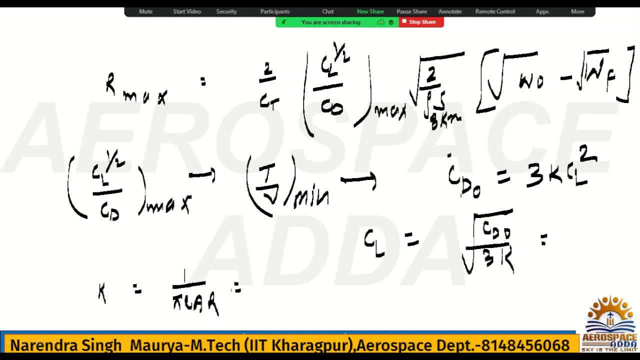 Yes, they have given the value. What value they have given to you? Check that. what value they have given to you? k and this 1 upon pi, Postval efficiency. they have given to you 0.87. and what is the aspect ratio? It is 6.5.. So if you calculate how much you may get, How much you may, 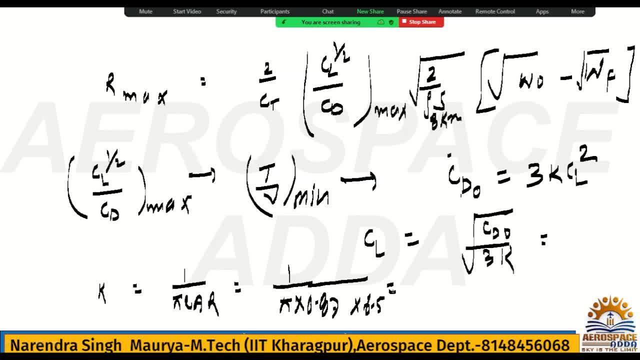 get 1 upon pi, divided by 1 upon pi, divided by 0.87, divided by 6.5.. It is, I think, 0.056.. And what is the CD naught in the problem? they have given 0.032.. In the problem it is given, please read that 3k k is nothing but 0.56. 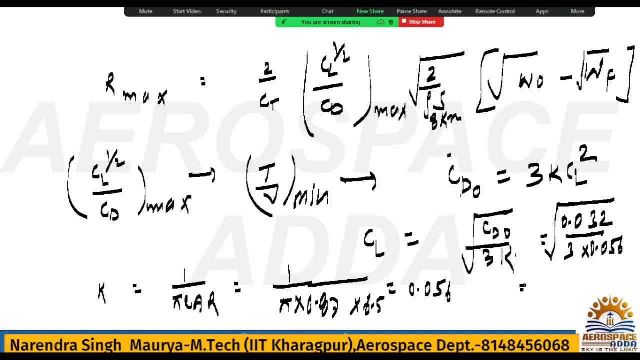 So this is the CL: How much, If you calculate okay, CD naught is 0.032 divided by this value. Okay, And if you take root of it, you may get check 0.435.. Check Quick. 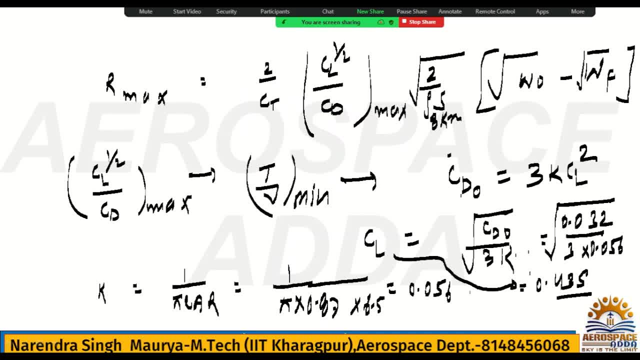 CL value. I am saying CL, Please go fast. 0.435.. Am I right? Yes or no? I think this is correct: 0.435.. Fine, So if you write CL to 0.435,, you may get 0.435.. 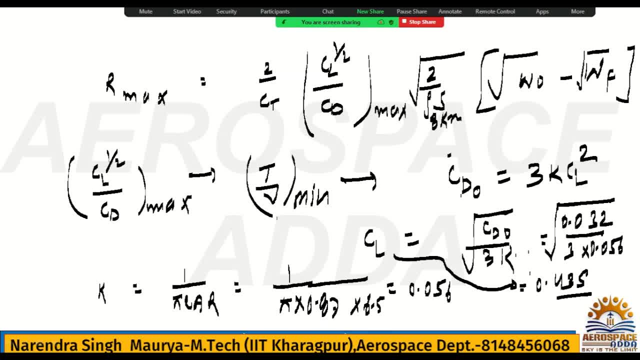 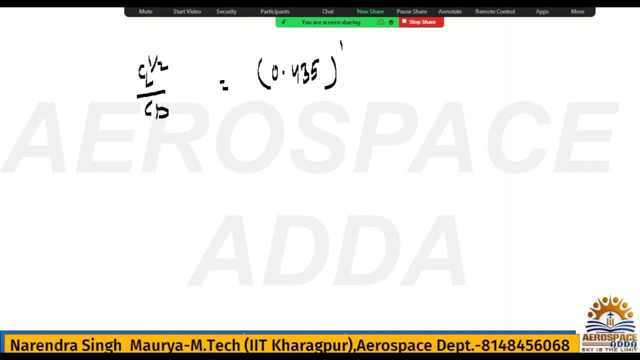 What is the CL to power 1 by 2 by CD value? What is the CL to power 1 by 2 by CD? What is the CL you have calculated? It is 0.435.. Is 435 whole power 1 by 2 divided by what? 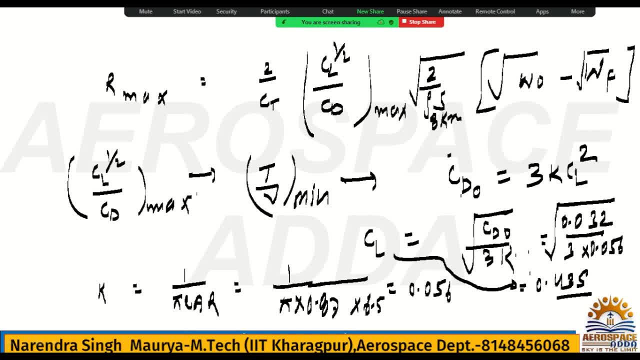 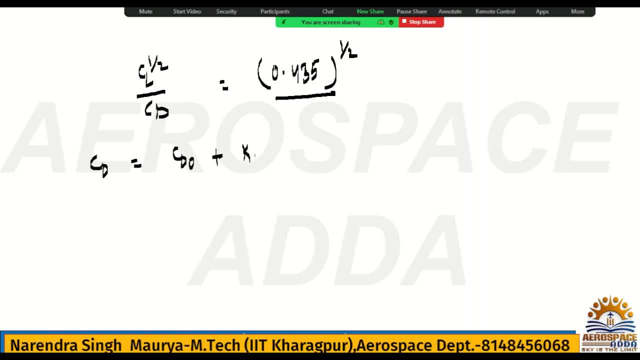 is the CD? What is the CD? If you remember, CD is nothing but CD naught plus 0.435.. So what is the CD? What is the CD naught? here it is given, What is the CD naught? 0.032 plus What is? 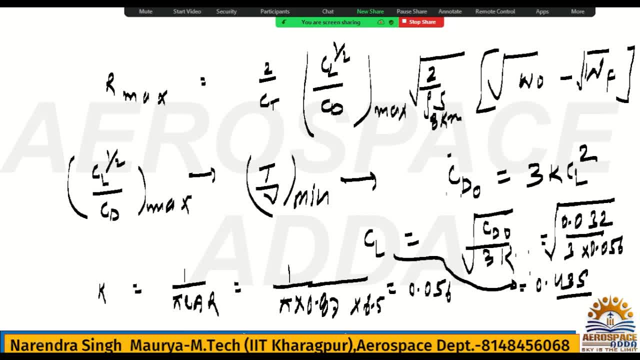 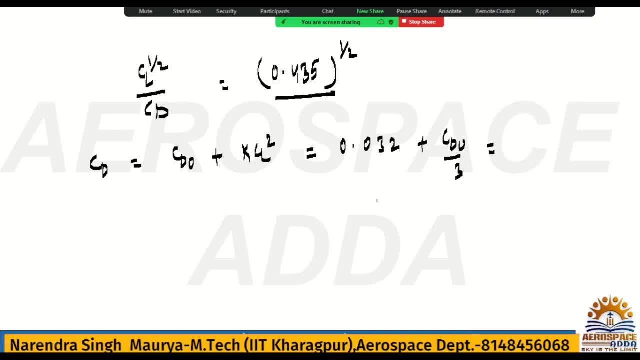 the KCL square Check. KCL square is nothing but CD naught by 3. CD naught by 3. So if you calculate it, so in fact here also you can write this better: This is nothing but what. 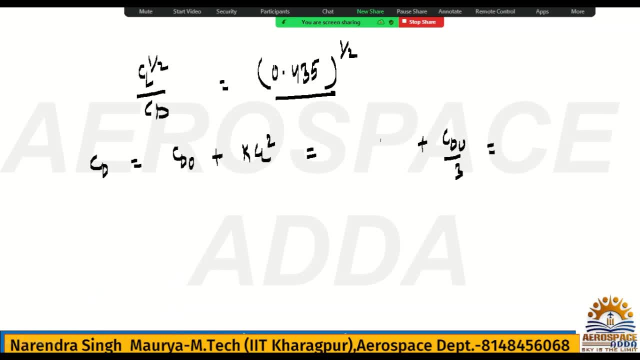 0.435.. So if you calculate it, so in fact, here also you can write this better: This is nothing but what. this is nothing but td naught, yes or no? so here you will get 4 by 3 td naught. 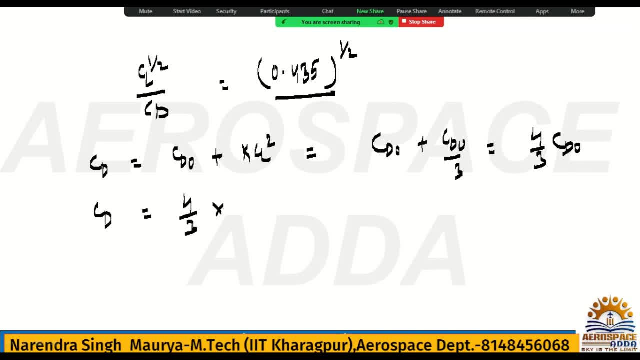 this derivation already i have done okay, so there should not be any doubt here why this is happening, what happening here. so don't think in that way, because already i have derived. so i am considering you guys remember that result. okay, if you calculate cd, then what value you may get. 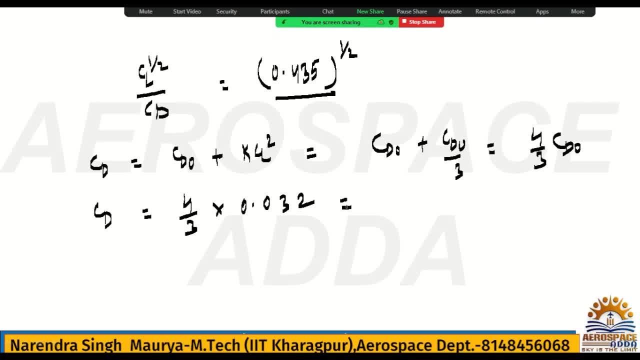 0.032. okay, 4 divided by 3, so it is nothing but 0.0426. now all the result: you have 0.0426. this now you calculate this ratio. i need this. so this is nothing but 0.435. it is nothing but check. if i am not wrong, then this result is: 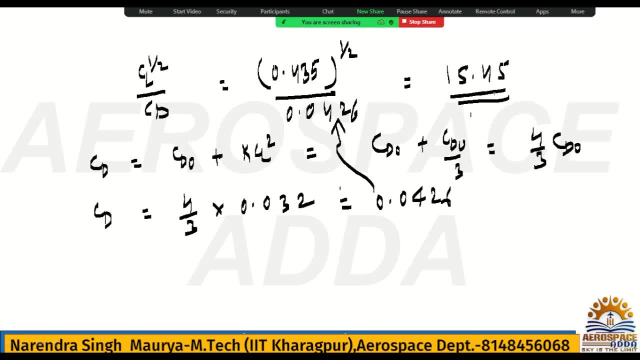 15.45. i am also calculating today because last class we had seen it was so much, you know, problem while we were solving the numerical. because calculation, your calculation is, i am thinking your calculation speed is what slow, so please go fast. it c? l to power 1 by 2 by cd. this is the maximum value you got now. simply, you just 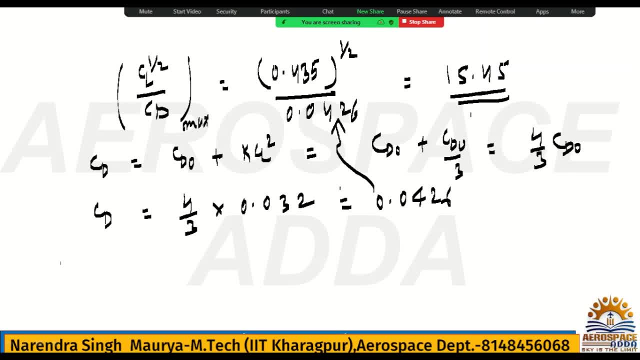 write all the results here. what is the formula? check next base. i will write again very fresh: r, max. what is that? 2 upon c? t here to power? 1 by 2. this is the 1 by 2. okay, and what is that 2 upon? 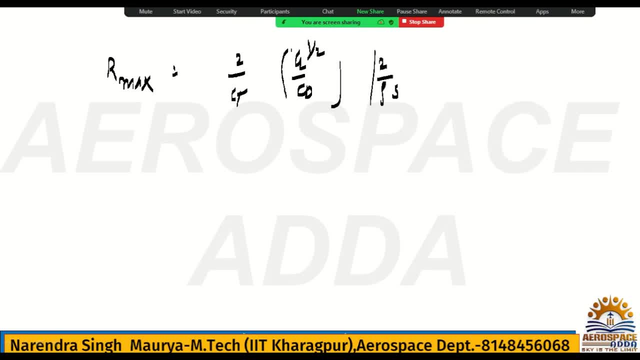 s know. Here, in bracket, initial weight minus final weight, Please write all the value 2 upon Ct. What was the Ct you had calculated? Check in your notes Just now. we had calculated that Ct is nothing but 2.78 into 10 to the power minus 4, equal to power 1 by 2 by Cdu. 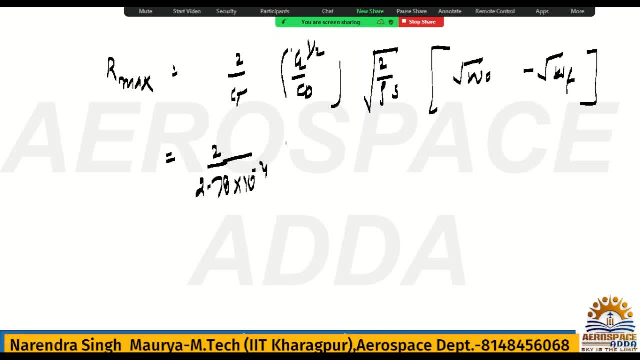 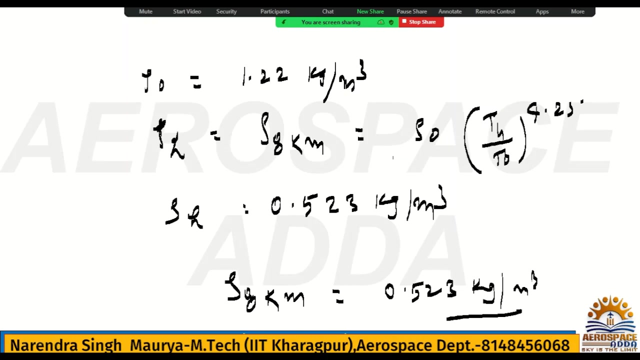 So just now you have calculated how much, It is nothing but 15.45.. This is the max value, ok, 15.45 in root 2 upon rho value, density, what you had calculated. Check At 8 km. you had calculated density How much: 0.523.. 0.523. 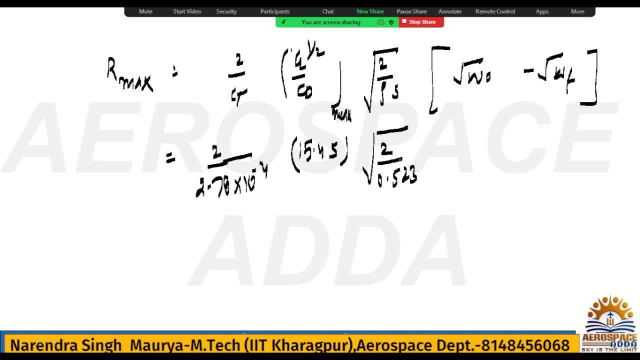 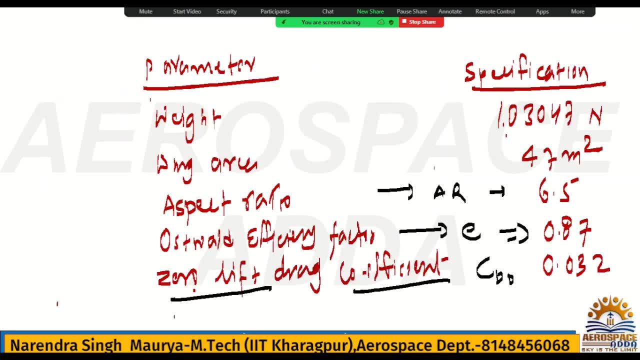 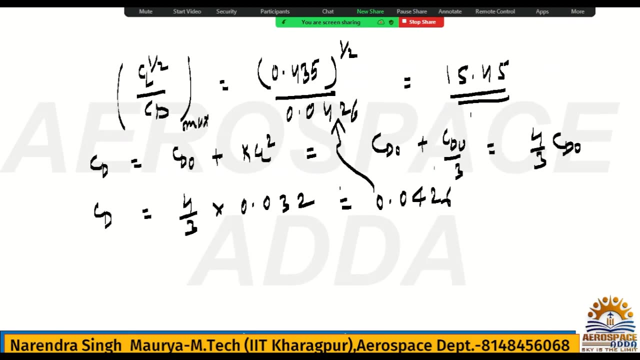 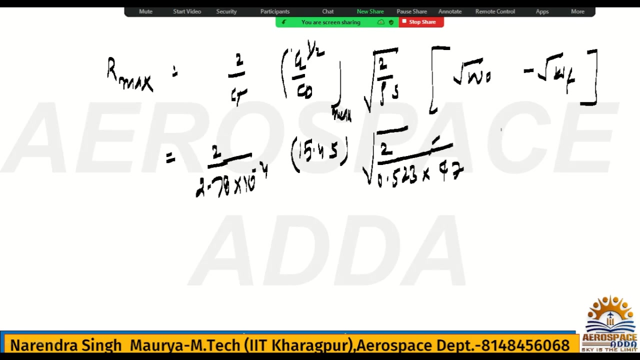 Into area, How much that area they have given to you. Take it, They have given that area How much: 47 meter square, 47 meter square, 47 meter square. Ok, Fine, Initial weight. What is the initial weight they have given to you? 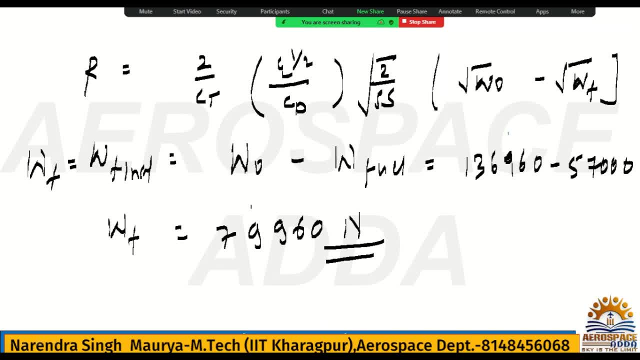 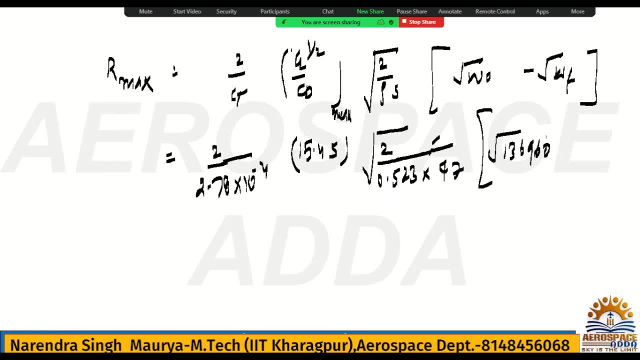 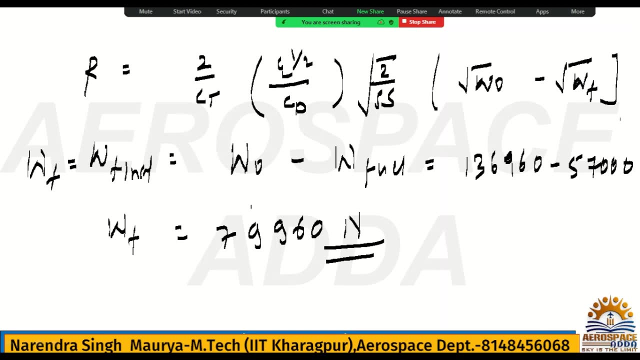 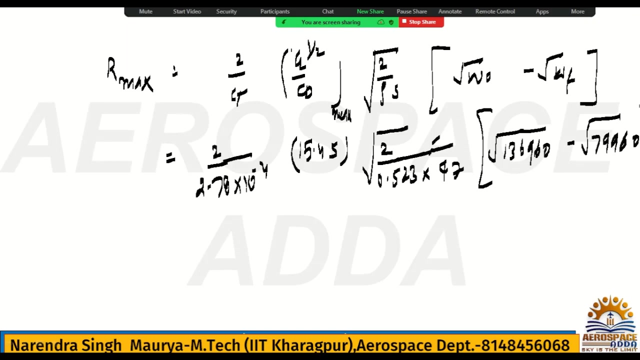 How much? 136960.. 136960. 136960.. This is the initial weight minus What is the final weight. Just now you have calculated how much: 79960.. 79960.. Ok, Now all the data I have written. 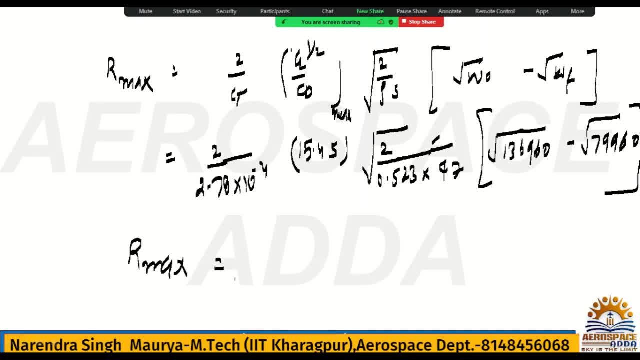 only you have to perform calculation, Use your calculator and get back to me How much you are getting. Go fast, Go fast. So if you do that, Then range you may get that is 3.65 to 3.66. ok. 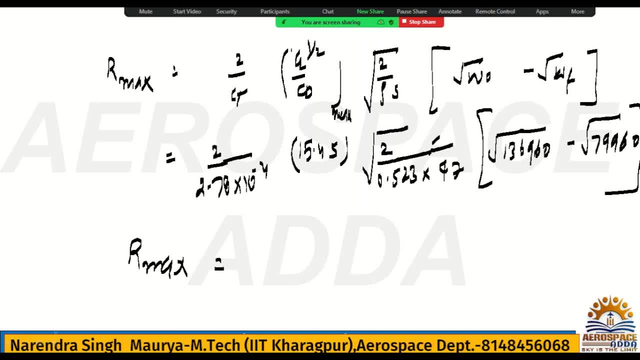 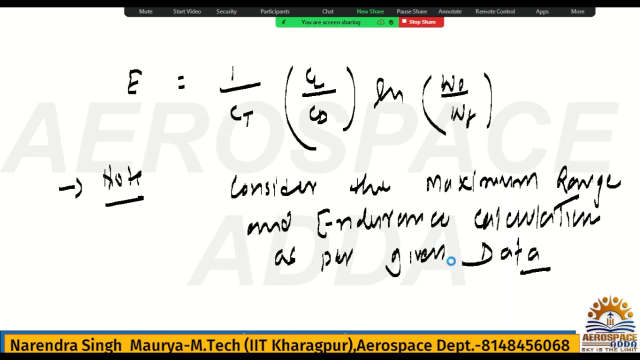 Then you will get, If I tell you that nearby, upon the calculation you may get a range nearby: 2.77, 10.6 meter. but if you check the answer here it is: it is given in kilometer, I think. see that unit now. 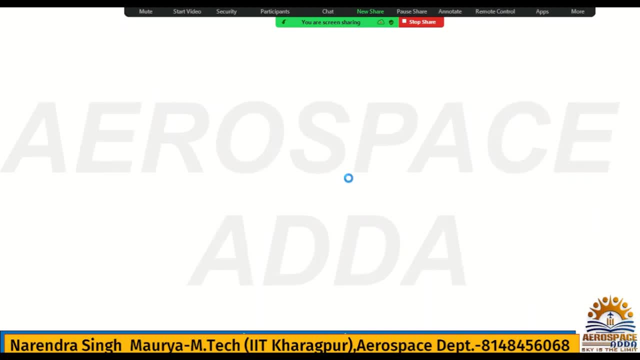 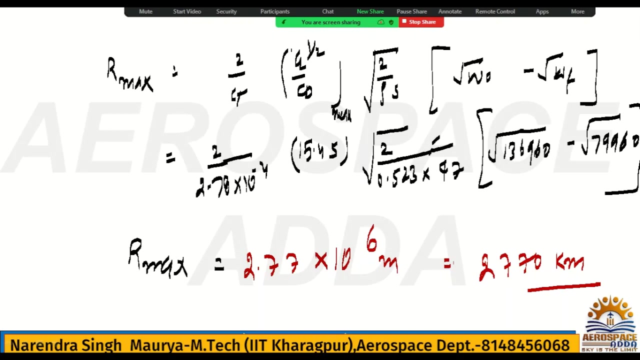 that unit is kilometer everywhere, so you write it in kilometer. so 2.77, 10.6. if you write kilometer, then what you may get, you may get 2770 kilometer. this is the range. okay, now we will go for the endurance. this is: 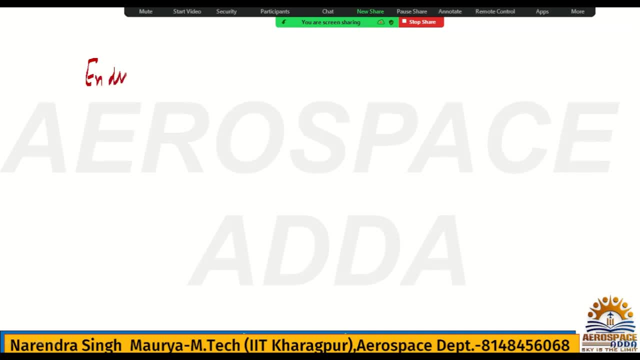 the range. please calculate endurance similarly. endurance maximum you will calculate. okay, sometimes in problem they will not tell you it is maximum or minimum, but you have to consider. all right, so you need to write 1 upon TT. okay, CL by TD, max. fine, LN. W0 by W0. how to calculate? 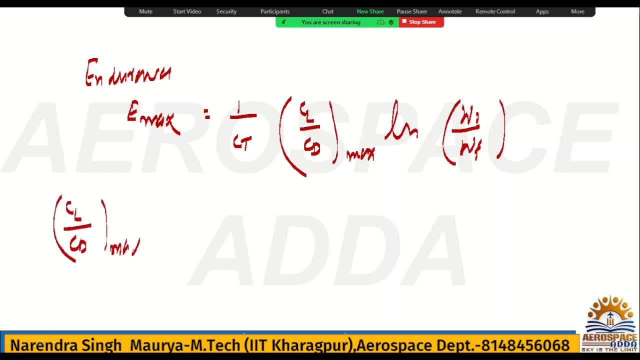 Cd max, fine LN W0 by W0. how to calculate Cd max, fine LN W0 by W0. how to calculate CL by CD max. so this CL by CD max is nothing but what minimum drag condition that you must aware about it. so what is the CLMD? 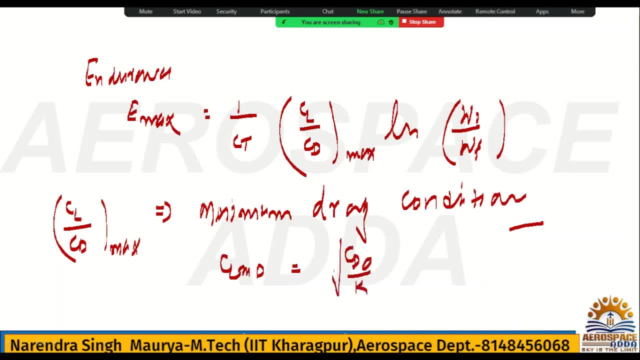 it is CD naught by K. yes, what was the CD naught? what was the CD naught? it is nothing but CD. naught is nothing but 0.032 divided by K. you had calculated- let me write here better- 0.032 divided by K. you had calculated K, yes or no? what was the value? 0.056. 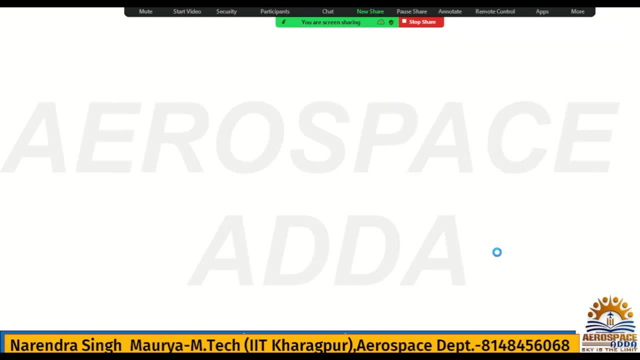 yes or no? what was the value? 0.056, 0.056, 0.056. if you calculate it, 0.032 divide by 0.056, you take root of you will get 0.75. now, what is the CDMD? it is 2 CD naught. 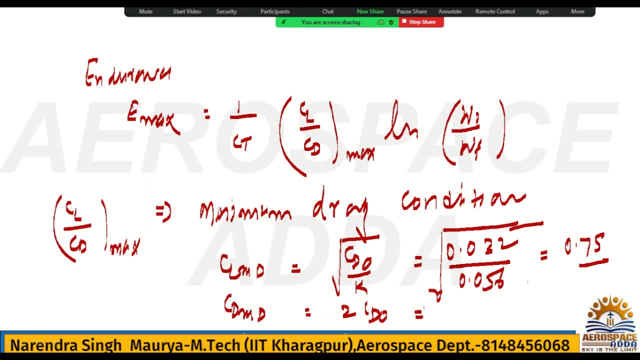 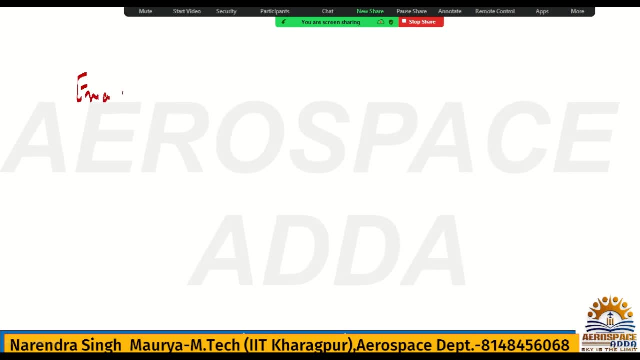 it is 2 CD naught. what is that cd naught? 2, 2 into 0.032. how much? this is 0.064. you keep the value here. okay, all the data in front of you now. 1 upon ct. what was the ct? what was the ct? check it was 2.78 into 10. 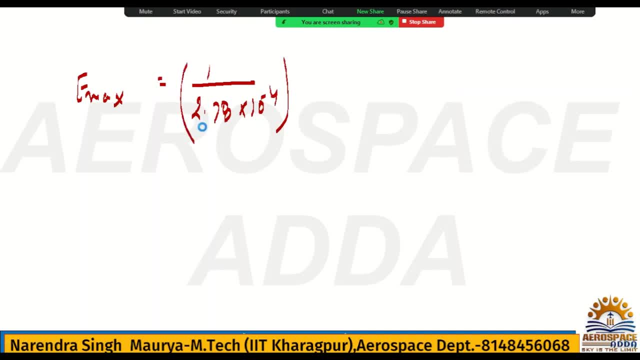 to the power minus 4. now cl. by cd you got. cl is nothing but 0.75 point seven five divided by zero. point zero six, four, zero six four. in the formula ln w naught, w naught was initial weight. what was the initial weight? one, three, six, nine, six, zero. 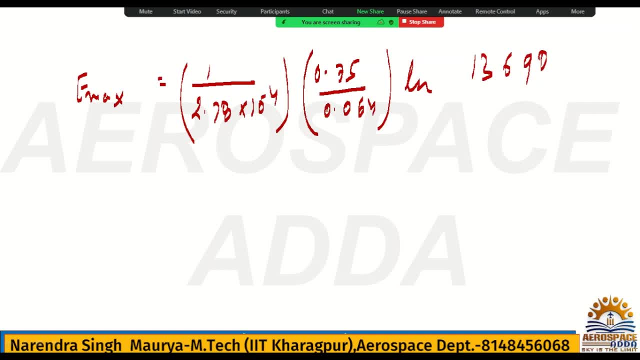 one three, six nine six zero. one three, six nine six zero. seven double nine six zero. seven double nine six zero. okay, now go for the calculation: one, three, six nine six zero, divided by seven double nine six zero, into ln 0.538 multiplied by 0.75. 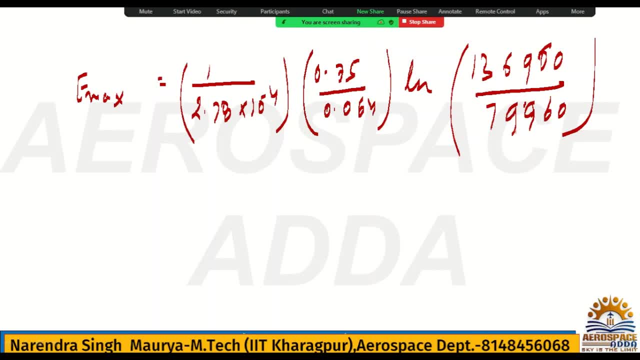 divided by 0.064, divided by 2.78, 10 to power minus 4. this is what i am getting. so so much to this value, but it is in second. we can calculate in hours. 2, 2, 685. i'm getting 0.57. remember ct unit you had calculated in second. this unit was in second now. 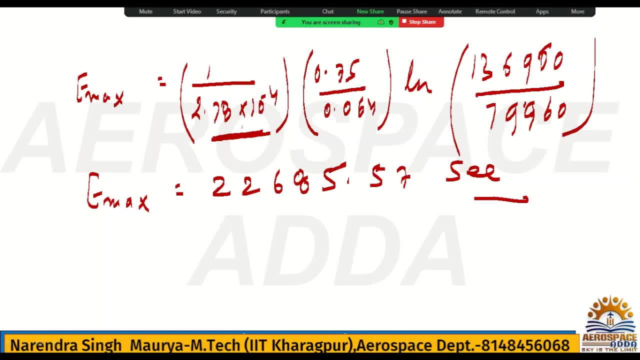 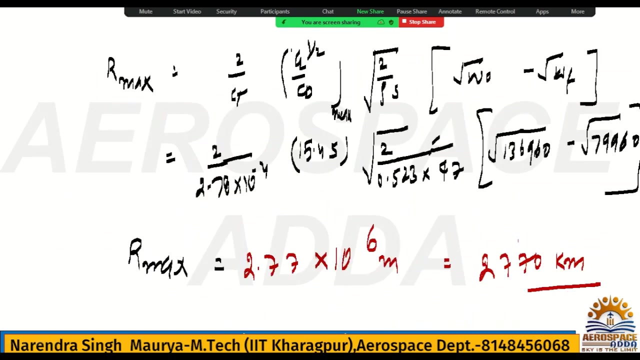 so this endurance is what? in second, now you calculate in hours. so what you will do, you will divide by 3600, so it is nothing but emax 6.3 hours. this is the one value. and what is the r max? r max, you got, check. two double seven zero. two seven double seven. 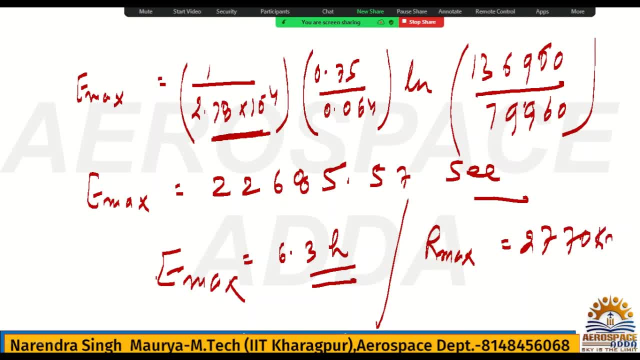 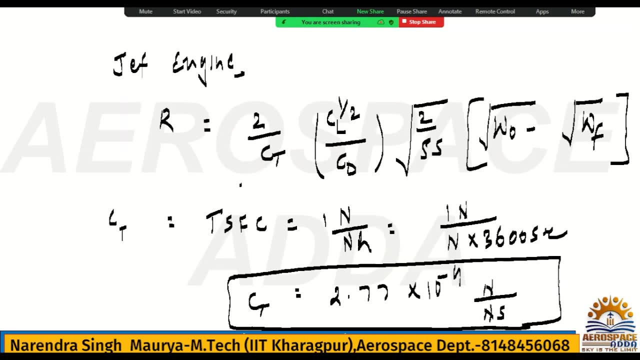 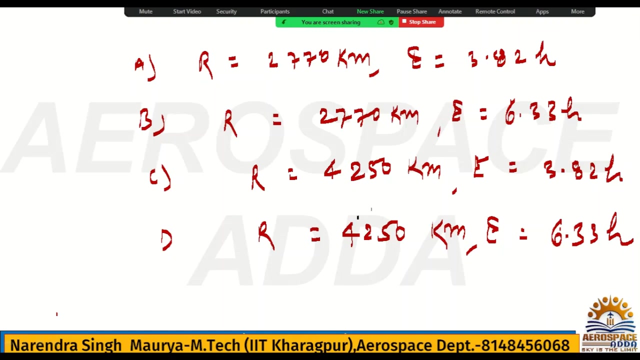 check the option now. what option is correct? take the option now where it is: see 6.3 hours. check here: 270 is here also and here also. but here, this is what wrong. this is what wrong. what is the 6.3? your option is b, yes or no. your option is b. 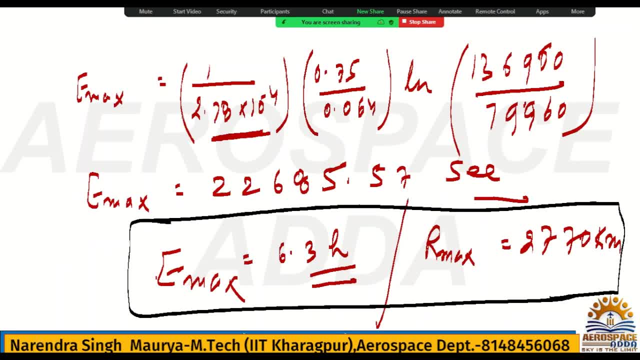 so b is correct answer. so you may think, like so much lengthy question, this type of question will not ask correct option. is that is true? this much lengthy question will not be asked to you. only one thing will be asked to you: what may be range, or maybe endurance. 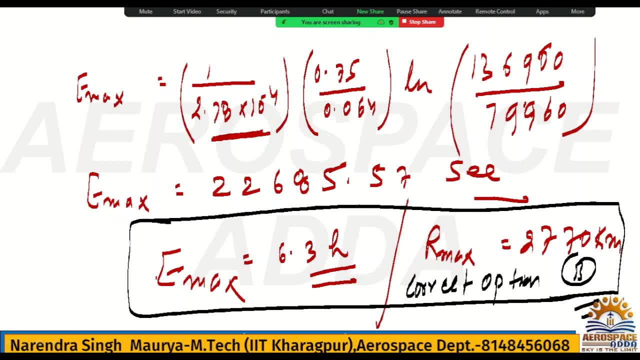 range. okay, maybe range or maybe endurance. they will ask to you so and all the data will be available to you in exam. i have seen what type of question they are asking. if this question will would be asked in exam, then you know what they will do. they will give all the data, only the thing they will ask, only endurance or 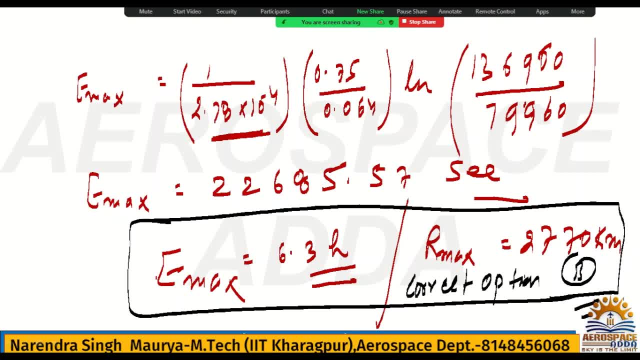 range everything they will give to you. in fact, sometimes they will calculate, they will give to you clmd and cdmd value also. or they may say like: okay, cl to power one by two, by cd maximum, is this. or they will say like: cl by cd maximum, is this that ratio also they will give to. 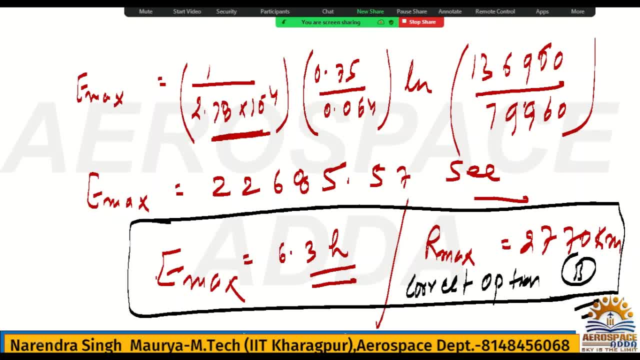 you sometimes because they don't want for two marks. you give 30 minutes or 20 minutes or one hour for one question. then obviously technically, if you think that is not possible, so whatever the question will be asked to you, they believe that within two to three minutes you can solve that. 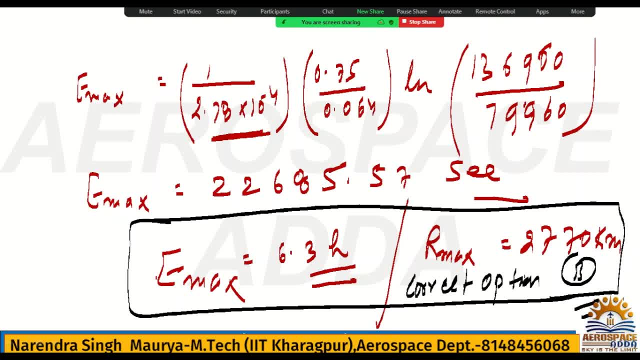 problems for two marks question, okay, so so don't bother. like okay in examination. if question will be lengthy, then what will? what we'll do that time i'm sure question will not be asked. read it if you think. okay, within two, three minutes i can finish. then i will do otherwise. you skip the question. 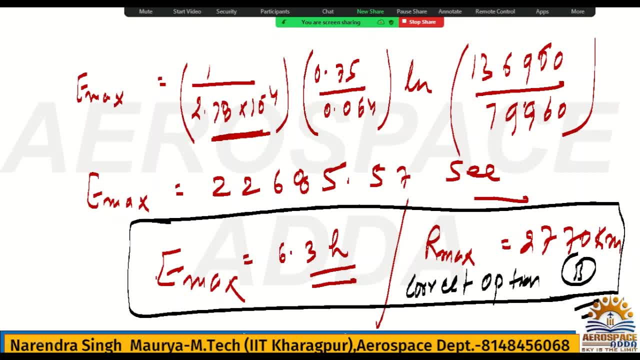 sometimes it happens very lengthy question they will give to you and solution will be lengthy. then you just skip that question because you have options. 65 question you have. if you solve 40, 45 question or 40 question, uh, properly you will be selected. so don't take risk in examination. 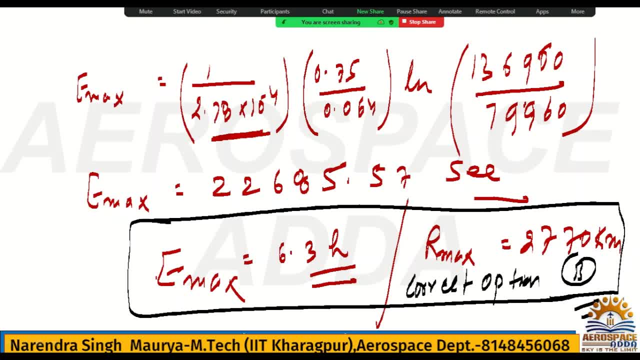 the question is very lengthy. sometimes they will go ask question in para. very lengthy paragraph will be there. so student may read two to three minutes. five minutes: they will read the paragraph. only don't waste time in such type of question. okay, that is the rejection of the question. selection of the question. you read it and you. 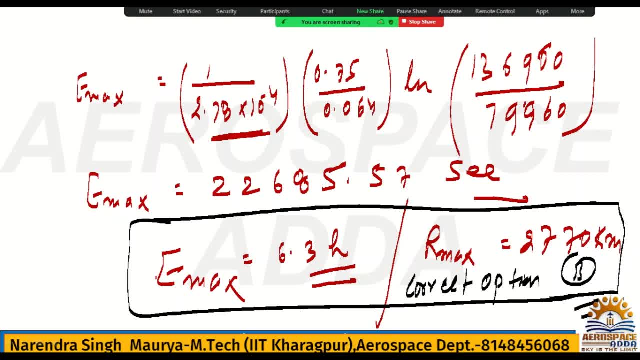 solve it. if it is possible, then you go for that. that is the selection of the question. you have selected that question. rejection of question means you read that question if you are thinking it is very lengthy, or sometimes it is calculation wise, it is really you are able to solve, but calculation. 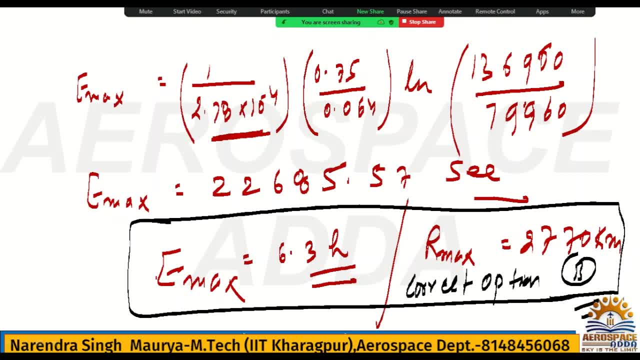 is: skip that question. that is the rejection of question. so in examination you have to be careful about it. okay, sometimes there is the plan in examination they may think like, okay, you will waste your time here, so they will do that question so that you can waste question will be very easy. 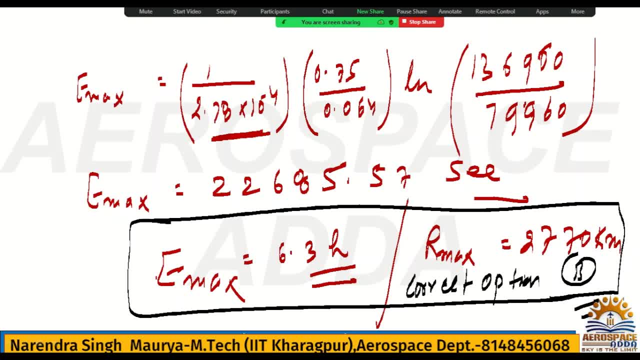 but that process will be very lengthy. so examiner, they are thinking they are asking you to solve that question so that you can waste your time. so be clever that time. okay, be clever and be smart that time that reject that question. i, i will suggest you reject that. why. 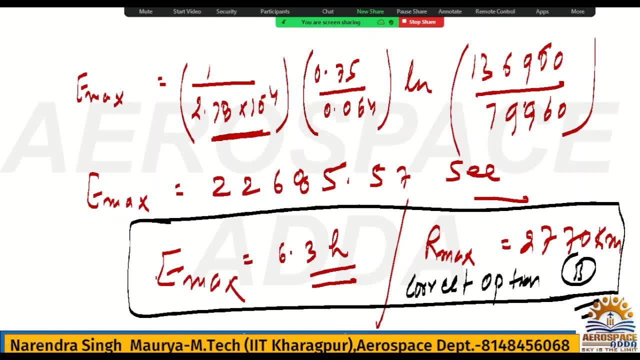 i am suggesting you because i know total question are 65. so if you skipping such type of question, one or two question, or 10 question also, or 15, 20 question also, still you have uh 40 to 45 question in your hand and that is more than enough for your selection. hope you understood all right. 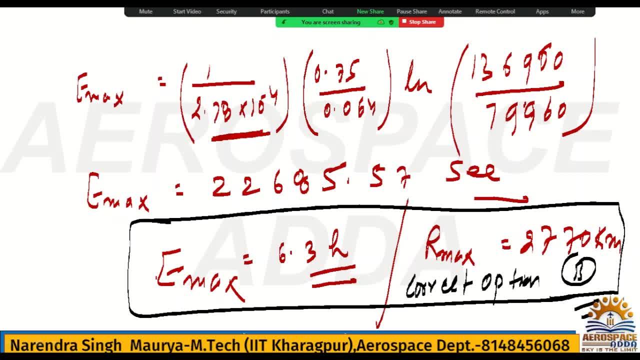 so these are the things. now we'll go for the next. okay, so this problem you have solved right, this problem, you have solved this should not be any confusion. there should not be any confusion. and uh, one thing i had not given, so you please make one table. so i'm just mark up this table only. okay, for range and endurance, for 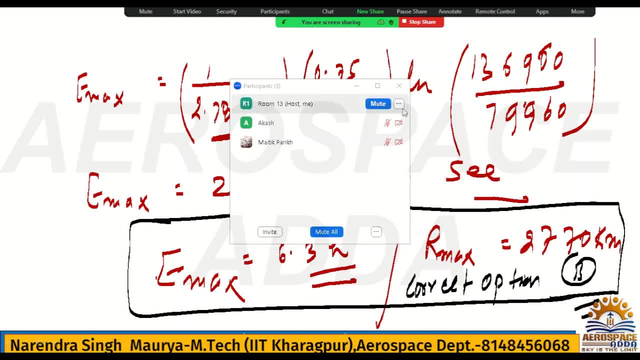 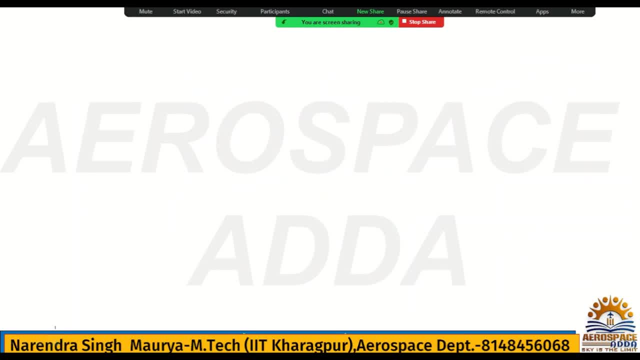 range and endurance. just mark up this table so it will be easy for you. fine, now right, uh, endurance, and this is what range? okay, you are talking about crystal engine or popular crystal engine. what is the formula for it? it is if propeller efficiency, like in one numerical we had shown. uh, we had solved last. 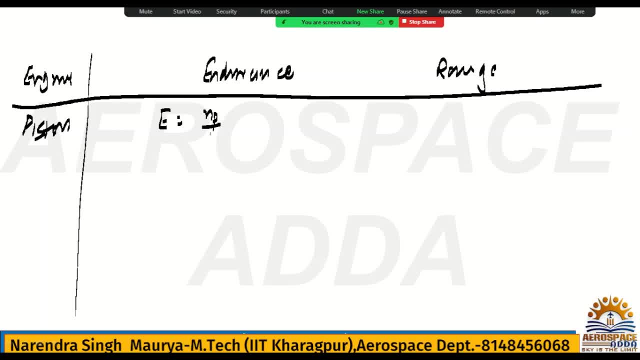 lectures. that was a popular efficiency was given. if uh, propeller christian or propeller no christian propeller, better be right, full popular propeller engine. so propeller efficiency they have given, then you multiply by eta p. if it is not given, take one, okay, cp and two row s okay. 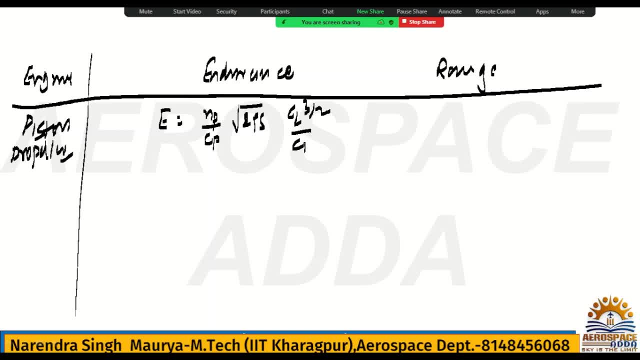 tl to power three by two by cd. okay, then it is nothing but final minus. initially. this is the range for what? the endurance for the endurance for the question. okay, remember, if they are saying e max, so e max will be field or response line. okay, kind of must. be balance, okay. okay, remember, if they are saying e max, so e max will be field control range your own. for course that is important, for the ship is like the receivers. the Attorney in the field can't care enough of غدель, of gold, and scrap as many rupees you can get in the dominating exchange field for trigger. 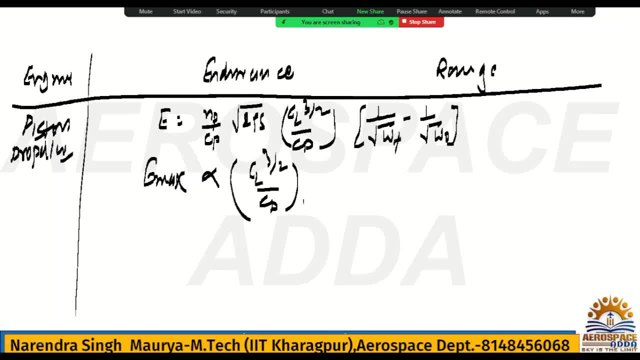 range for which will surely publish the smart sóloop. we are in science, okay, all in to math island and scantling for the power. 3 by 2, by Qt, This will be the maximum, Okay, Okay, And that minimum power condition. you know What is the minimum power condition? This is the minimum power condition. What? 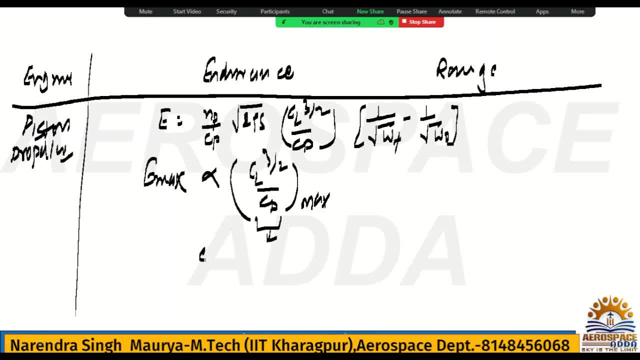 is that It is nothing but Qt naught is equal to 1 by 3 plus real square. This is the condition that you must aware about it. Okay, This is what This is nothing but piston engine endurance. Similarly you can write for jet engine also. I would suggest you make by your own, because 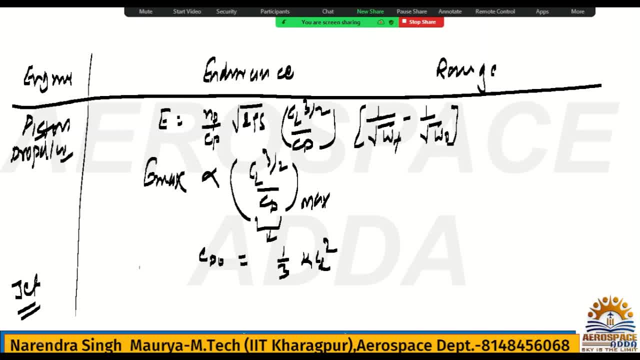 all the formula you have. it is given to you. So similarly you write the endurance formula for the jet engine also. What is the formula? 1 upon Tt? Okay, Tl by Td, ln. Can you say by final Yes or no? This is the formula for the jet engine Here also, if maximum. 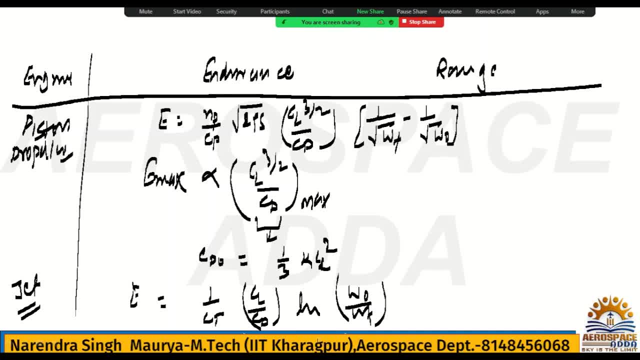 endurance they are asking. then Cl by Zt should be maximum means minimum drag condition, Yes or no Minimum drag condition. Similarly here for the. you just make proper table and remember this formula. only I would suggest, do not go for more and more numerical, because 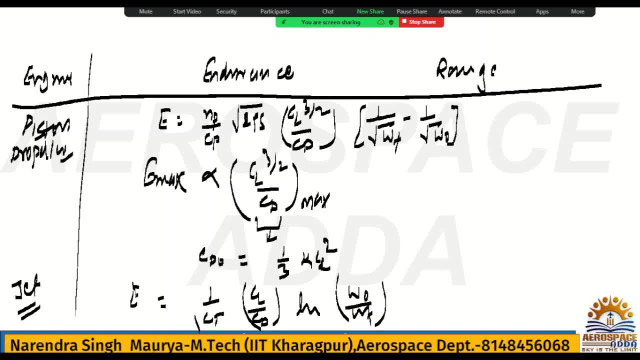 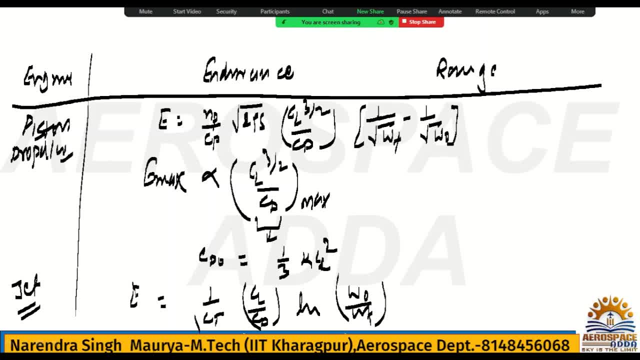 formula. that is very important. so now, 2-3 problem you have solved, so you are now ready to apply the formula. now your important job is to remember to mug up the formula. so for that I would suggest you to take a big page and write formula properly. okay, maximum minimum. 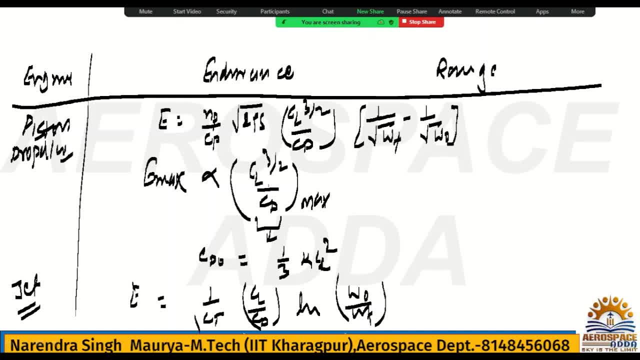 condition and write the endurance and range formula first of all and you mug up it. okay, so what will be the piston prop range? that formula will be eta p again, propeller efficiency divided by CP. okay, c l by c, l by c, d l n. it is nothing. but W naught by W? l. this is. 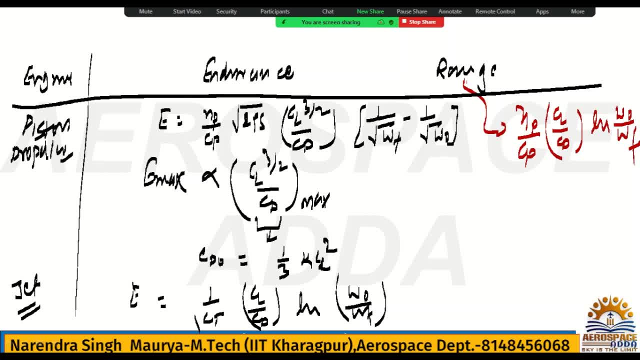 a formula for the range. similarly, if you go for, you just make the one page and remember this, okay, and another formula is nothing but for the jet engine, that endurance will be 2 upon you. just now we had solved that: 2 upon c, t elim to power, c? l to power, one by two. 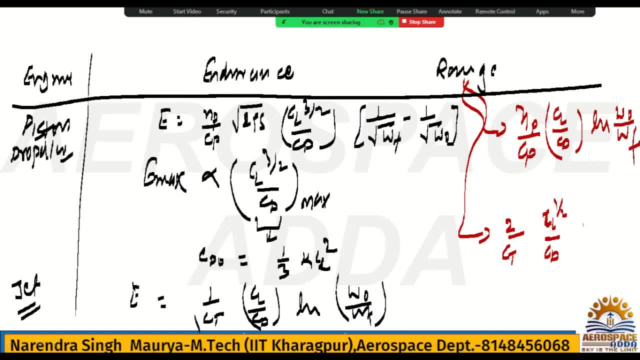 and par nine. I must write here CL upon 1 by 2 by CD and 2 upon rho s. just now we had solved problem. based on it, it is W naught, initial minus W. So just make one table and write the condition. 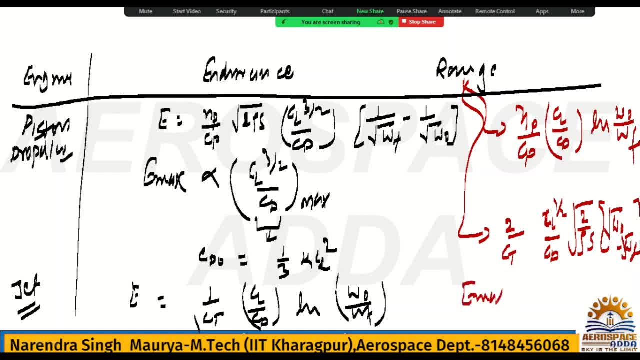 if you are going to calculate, suppose, E max for this, then E max will be what CL to power, 1 by 2, by CD max, and this is nothing. but what is the condition here? you know that CD naught is equal to 3K, CL square here. what is the condition for this? CD naught is equal to 3K. 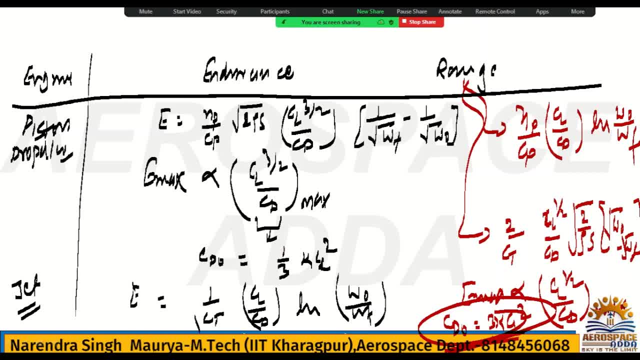 CL square. So this: if you remember this, only this condition. if you remember, then only you will to hit the question, otherwise there will be difficulties. okay, So please be aware with this. there should not be any confusion about it. So I think range and endurance test problem. 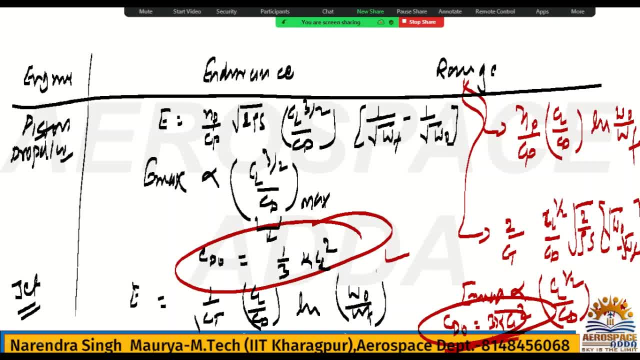 we had seen 2-3 problems we had solved. still, range and endurance required in range and endurance problem will be solved if it is required. then again we will solve it, okay. So now I think we should stop this range and endurance topic. we should go for the other one, yes or no. So now you are knowing that. 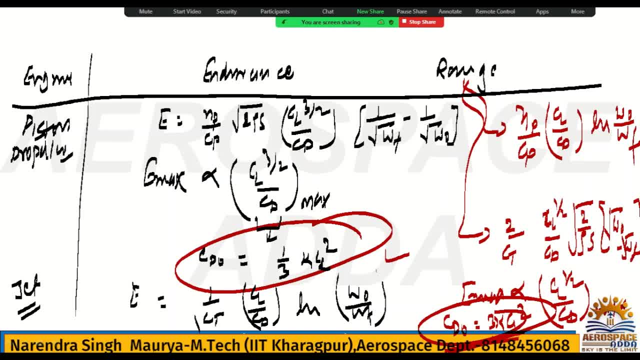 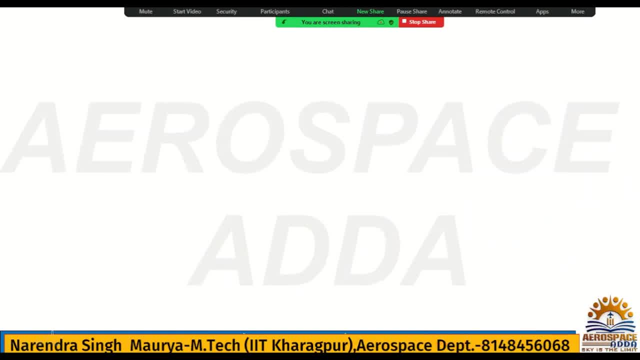 types of range. I would suggest you: what is the types of range? So types of range. basically this is the theory part, but yes, I am thinking some maybe it is asked. so then theory part also. sometimes they are asking, so you should know types of range. 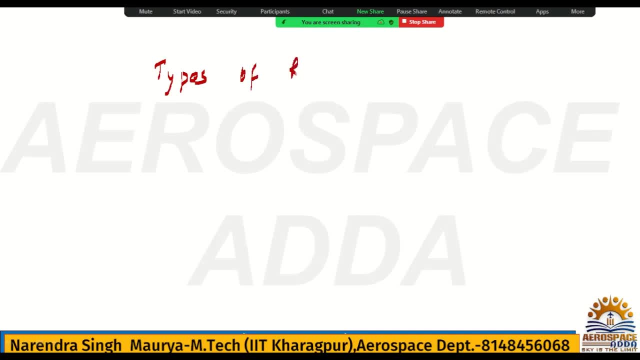 give a heading, a very small heading, types of range. okay, types of range. So here if you talk about the types of range in short. so I will explain by the diagram, it will be easy for you. So this types of range, we have three types. it is called SAR: okay, safe. 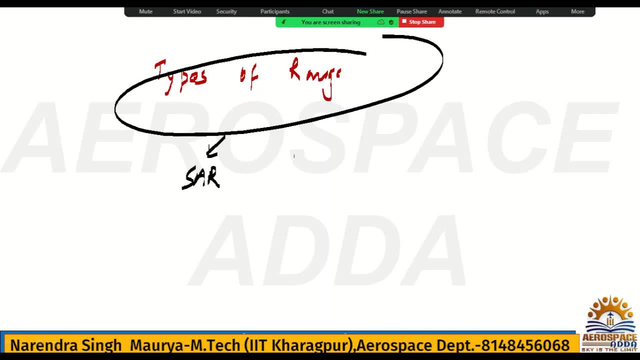 safe air range. another is again it is called: this is much right, safe. again it is small sa. or I can write: still air range, still air range, okay. third one is still air range, then GSAR. it is nothing but gross. it is nothing but gross, still-air range. 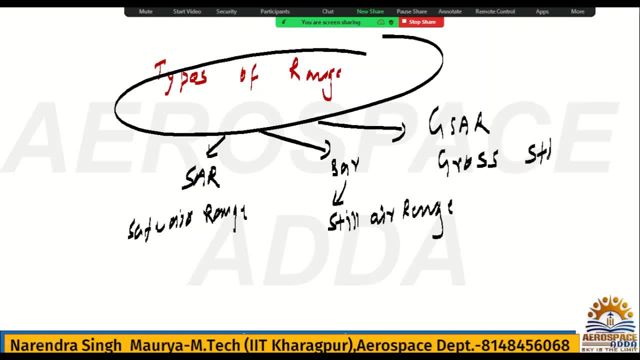 So, don't worry, I will explain here. don't write anything, right? yes, draw the diagram. I will draw the diagram there. I will explain: still-air range. these are the 3 types. okay, Number 1, 2, so sometimes if they ask the solution, double time problems, if they mention it, then you. need to answer that. So if you know this, it means you are going to make a discussion about these. Some of these are burner channels. okay, then you can do these types of jim mass diagnostics. these are the two most important types. the difference between a 79 and 大 proud of affects is always clear. 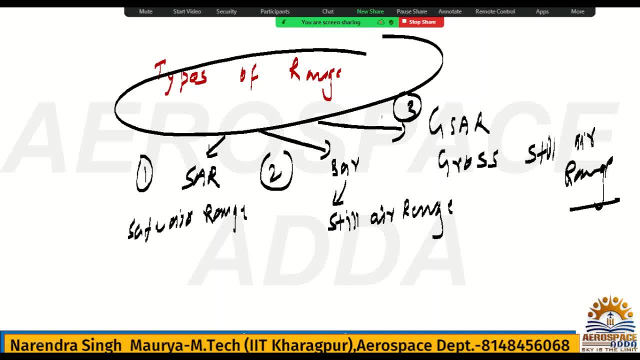 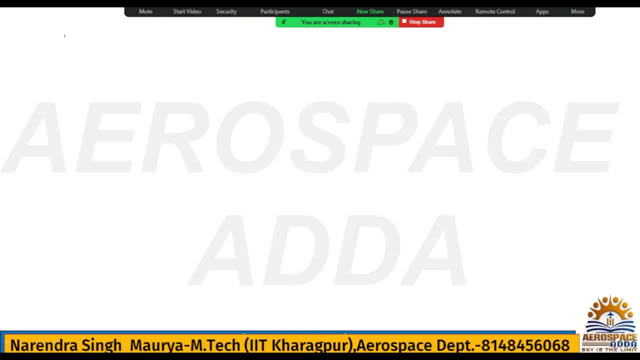 send it, then you need to answer for it now, yes or not. now we'll go for the diagram base analysis, so that will be easy for you and, in short, we can finish all first. one is nothing, but it's still a safe area- sorry, safe here- which is called s, a, s, a, r. all right, what is the sar? so you check the. 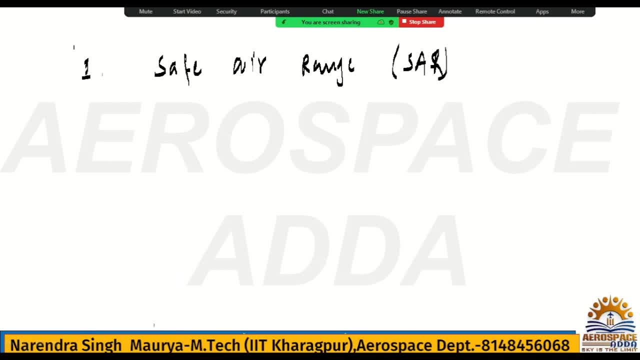 diagram. by the diagram only, you will understand. it is the maximum horizontal distance. listen carefully. it is the maximum horizontal distance that the aircraft can travel safely, which considered the amount of fuel required for each segment of flight, which includes takeoff, climb, cruise, glide and landing. that will be called as a safe air range, if you talking about the chip. so 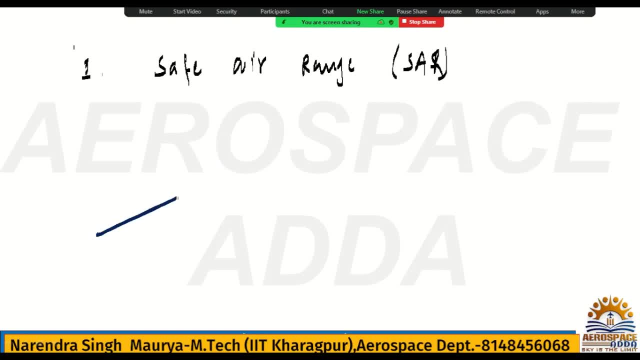 diagram. you draw it here. that's, that's all. this means it's a very long distance and the for Tôi peace loop, you know, underneath this 10 it shows slightly distance. okay to check. this is called take off, this is called climb, this is cruise, this is called. 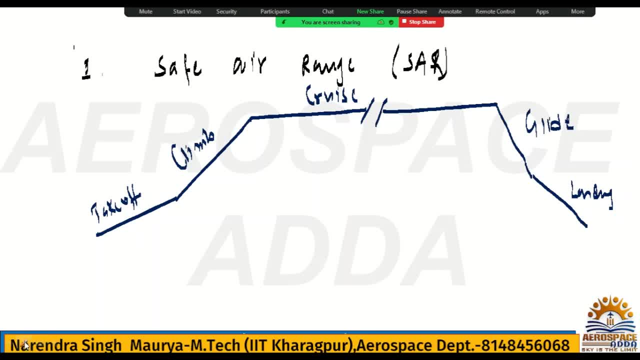 glide and land. this is the whole distance. so if you talk about the safe air range, so this will be the safe air range. SAR okay- means it includes all, it includes take off. so SAR, SAR means safe air range. it will include all: take off plus climb, plus cruise, glide plus landing. 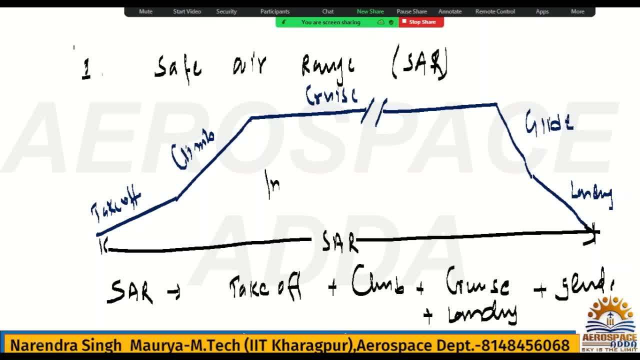 this will be called: includes all must ride, includes all operation. this is called safe air range. again, i will tell you it will consider the amount of fuel required for each segment of flight, which includes take off, climb, cruise, glide and landing. so this whole distance will be covered from i. 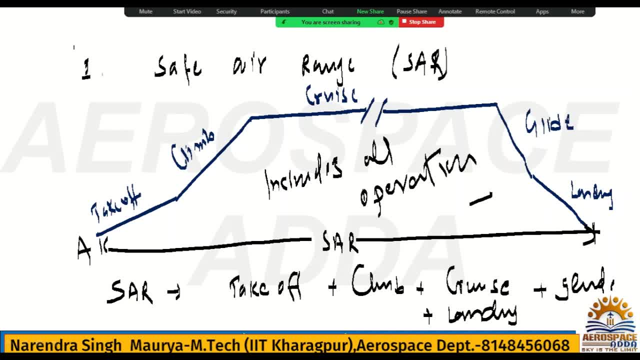 can say this is nothing but a to b, then this will be called as a safe air range. hope you understood. this is the diagram only you draw, so you will understand. okay, it's very interesting thing. the thing is: go for definition. don't write definition. better, you try to understand by the diagram. so second, 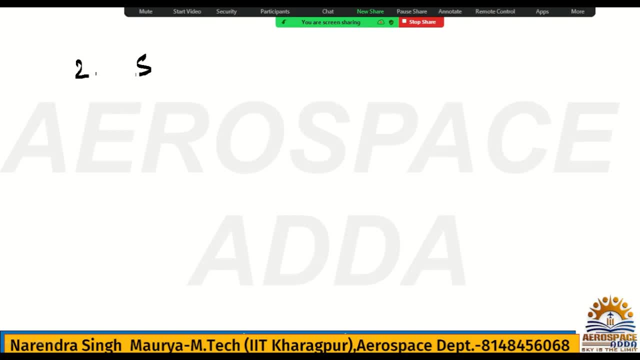 one is nothing, but two. what is this? is still air range small is air. what is that? again, i will do the operation to you so it will be easy to understand: check, take off, client, and this is going to okay. so now see, i think this diagram i have not drawn well. 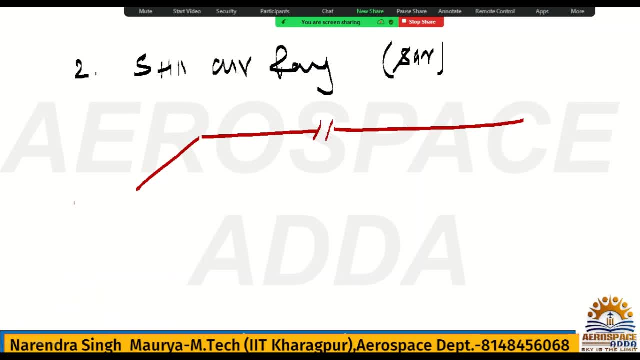 should be little bit. ah now fine, so this is what take off is fine. so so range means only till cruise. you have to consider then what distance it is covered. this will be called as still air range. it is not safe air range, it is still air range. so this distance, 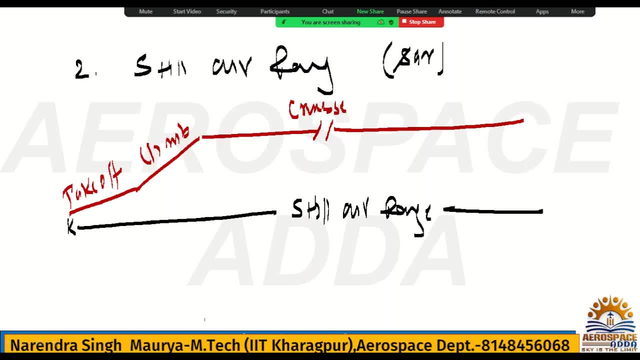 travelled, this will be still air range. here you are not considering gliding and landing, so this is small as a r, which mean still air range. includes what take off, climb and cruise, then it will be still air range. draw the diagram: whatever what you have take off, climb and. 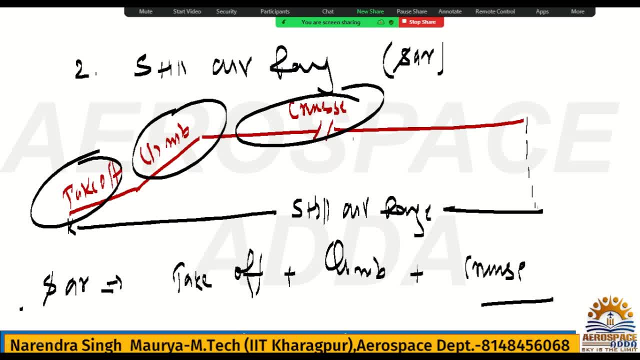 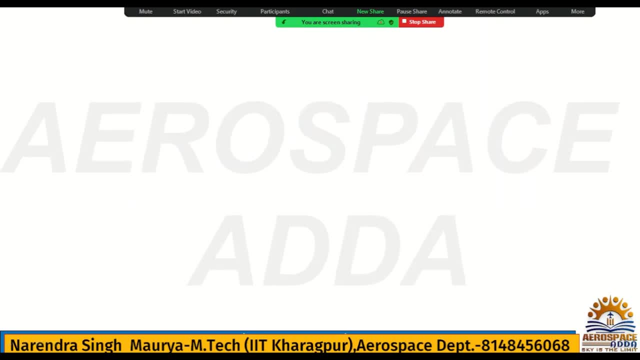 cruise, then for this distance, whatever amount of fuel you are carrying, so for this operation, only takeoff, climb improves, then it will be called as a still air range. okay, now we will go for the next. now we will go for the next. what it is? third one is nothing but gross, gross. still air range, okay. 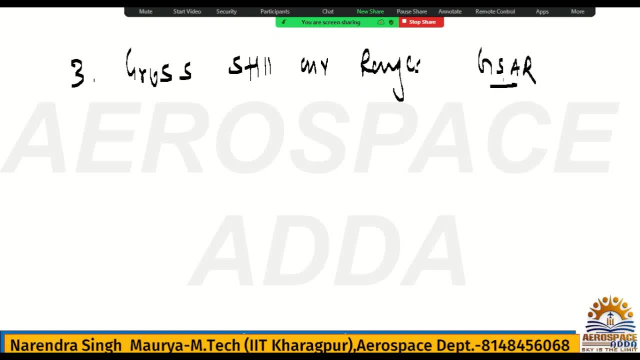 this is called gs. what is gsar? listen carefully if you talk about the gross, still air range. so that means the aircraft is assumed to be at a selected altitude, means it is reached at any altitude. suppose this is the aircraft. it is selected, any altitude it is from the sea level. suppose this. 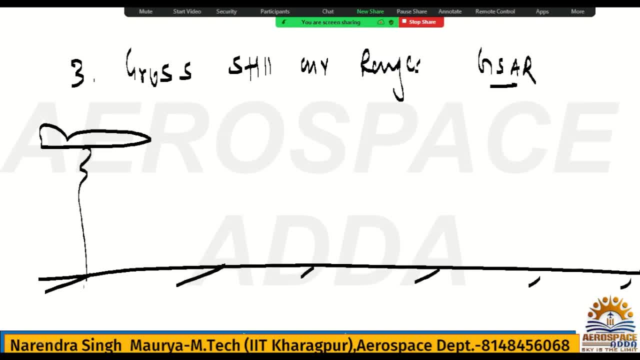 is the sea level. it is selected any altitude, just say it is suppose eight kilometer. okay, now what distance? okay, fine, aircraft is assumed to be at its selected altitude. at which cruise is starting? at which cruise is starting? i am saying, cruise is starting from here, only let me give another color. 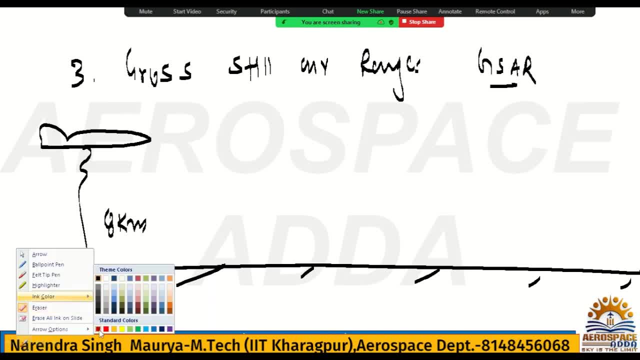 so it will be more clear now. suppose cruise is what is starting from here. okay, cruise is starting from here, only so, oh my god, so color, right. so cruise is what is starting from here. fine, it is starting from here and it is going for a long distance and it is. 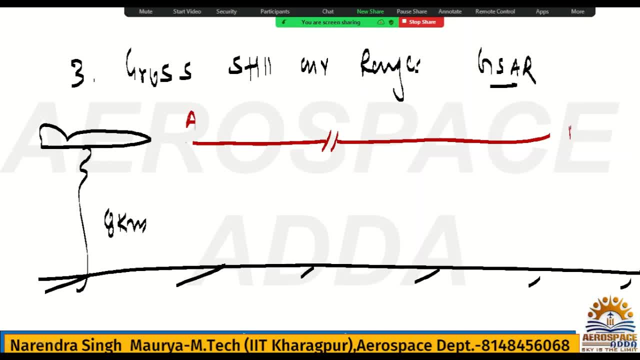 ending. so this is the cruise. cruise is starting here and cruise is what? ending here. so this distance, okay, the aircraft is assumed to be to be at a selected altitude. i am selecting it is at kilometer altitude, which cruise is started with full- uh, full fuel time and full flying speed. 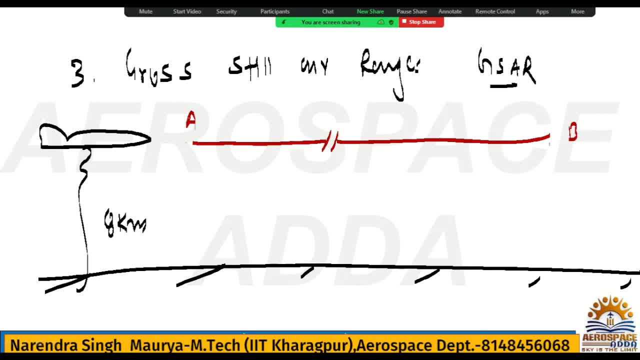 the takeoff and flying segment of flight are ignored, then the horizontal distance covered until all the fuel is consumed is called gross, still air range. so if you are, if i say what is the gross, still air range, so you have to say this distance, only this distance is nothing but called gfar. so that g s a r, it includes only crew. 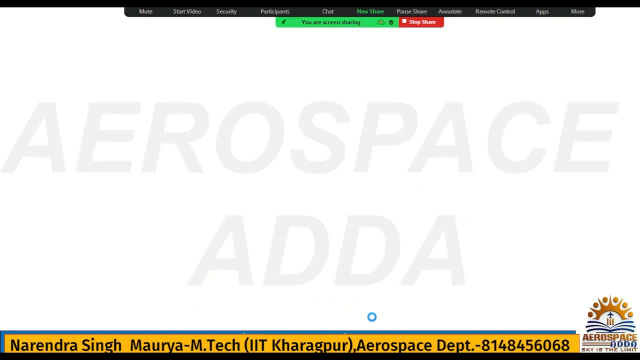 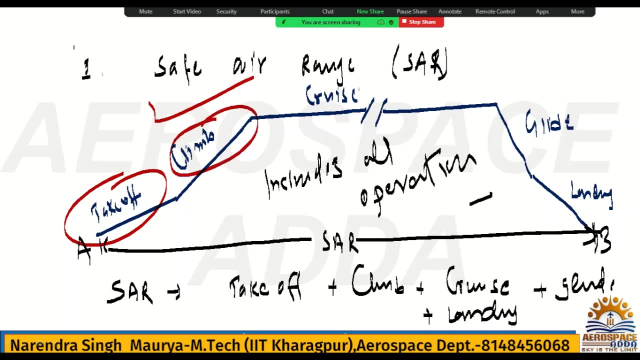 g sar. it includes only crew. g sar, it includes only crew. g sar it includes only crew. so if you check the diagram systematically i have explained. i mean first i have taken full all the operation where it was take off, climb, cruise, glide and landing, all the operation. if 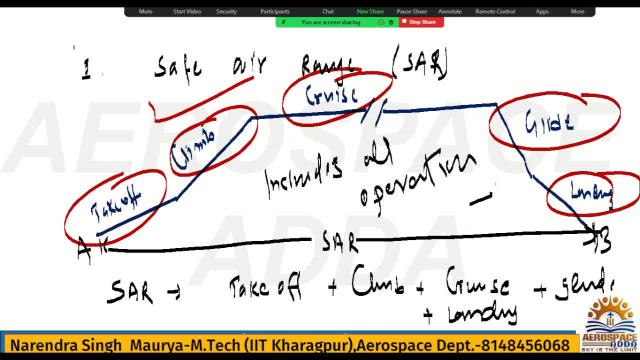 you take and for the full, full fuel tank. you are not going to refill it for the single filling of the tank. if this all operation, if you covered, then what range horizontally? what distance? maximum distance it is covered by the aircraft called safe air range. always remember it, okay, sorry. 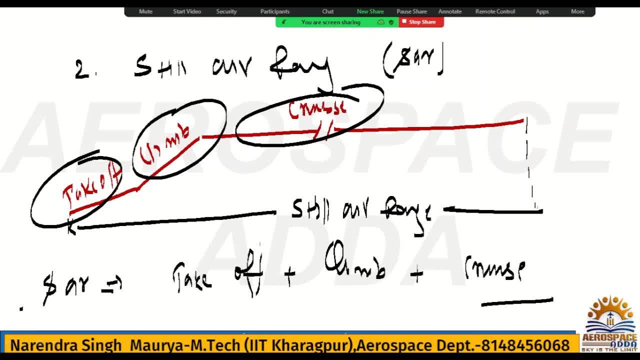 second is from the operation take off, climb and cruise. i have taken gliding and, uh, landing. that operation is what not considered here, if these three operation is what covered by the aircraft. so what is the macro horizontal distance that will be called still air range. third, here in this case,